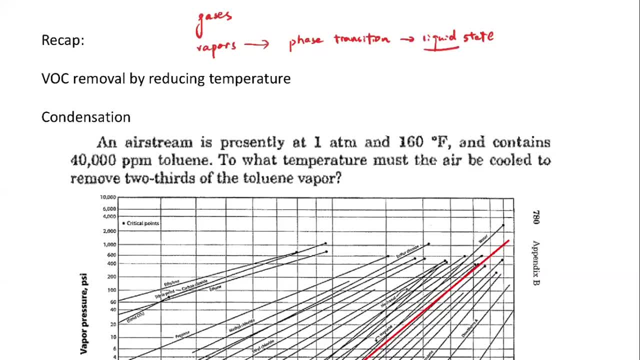 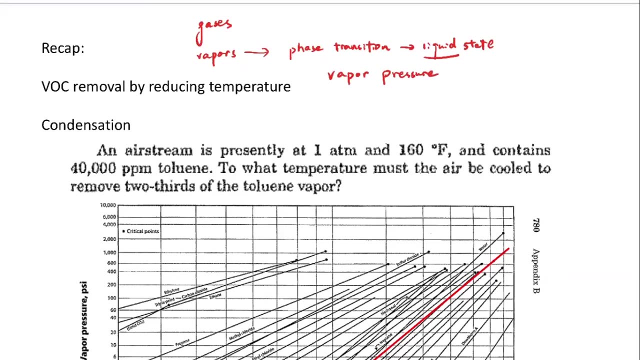 the liquid state in there And since we talk about the phase transition from the liquid to the gas, we introduce a very important concept which is the vapor pressure, So the vapor pressure. people also call them saturation vapor pressure. So basically this is the maximum. 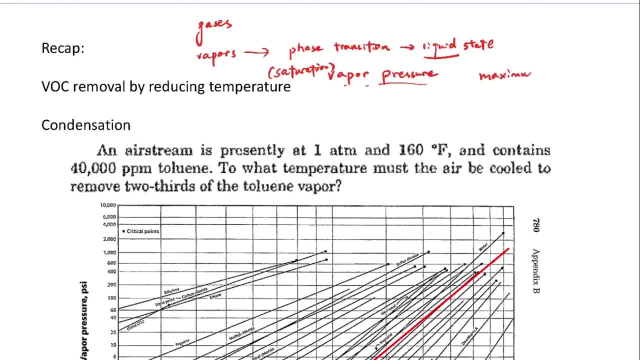 partial pressure, So basically the maximum partial pressure that this vapor can have. If it's above this vapor pressure, if the partial pressure is above the vapor pressure, then they're going to condense And that's why, for the relative humidity, the RH always. 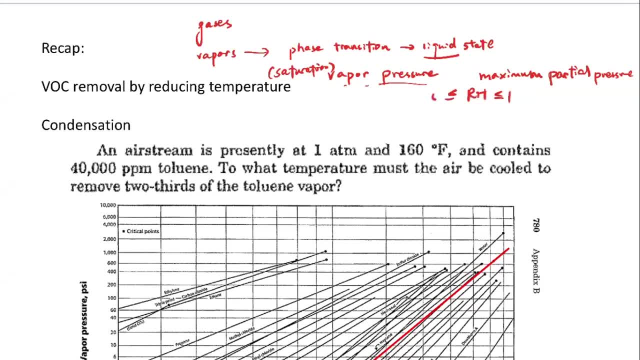 have to be equal or below one. Thank you, equal below zero, right? So there's no way that under equilibrium, the water vapor can be above the partial pressure of the water, can be above the vapor pressure of the water, And we also. 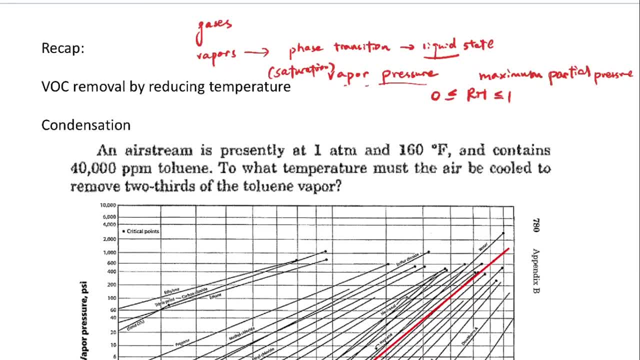 mentioned the temperature dependence, So we introduced the equation that's called the Antoine's equation Spell. that That's Antoine. So Antoine's equation basically tells you the dependence of the vapor pressure on temperature, which is PVI, equal to A plus B divided by C plus temperature. 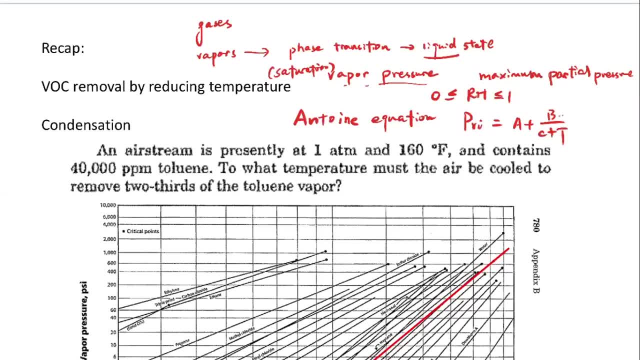 OK, We mentioned that the B term here is negative. So that's why we have basically a trend where the vapor pressure is going to correlate with the temperature. So just to know whether you guys are familiar with this, I'm launching a quiz. 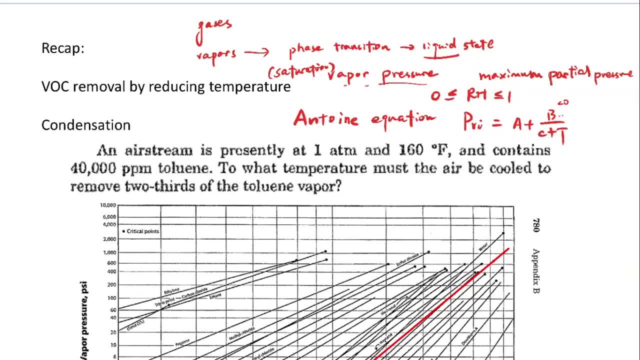 So how does the vapor pressure change with increasing temperature? I'll give it 10 more seconds, Okay, I will stop here. So the correct answer should be the first one, which is: the vapor pressure is going to increase with the temperature, right? 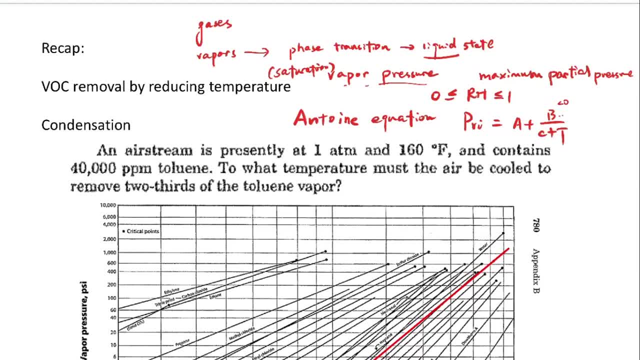 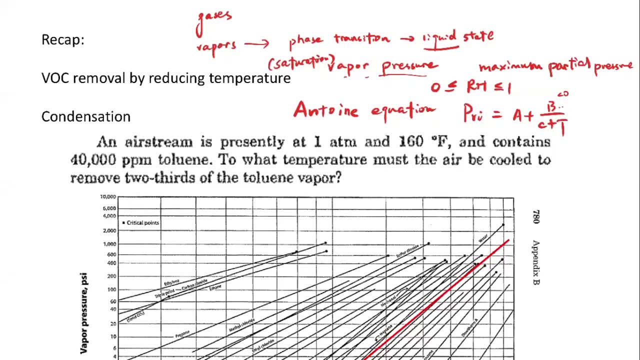 And we showed a video that demonstrate how we form clouds. So basically, it's a low temperature that cause the vapor, or cause these water vapor, to condense, right. What that means is under low pressure, under lower pressure, the saturation vapor pressure is lower. 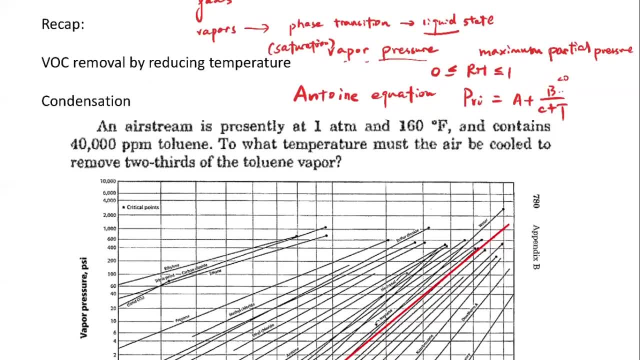 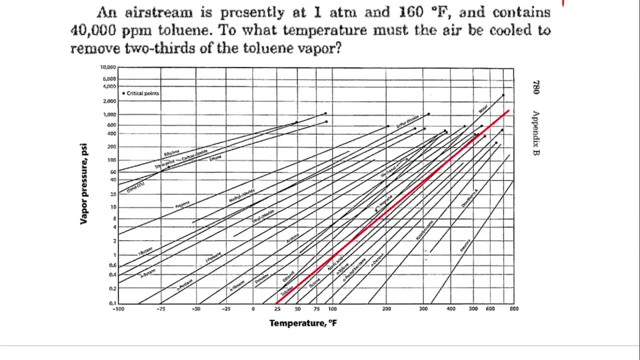 as we have the condensation right. So basically we have the relationship that the vapor pressure will increase with the increase in temperature, right? And so basically that's the Antoine equation, And at the end of last class we introduced that we can actually remove. 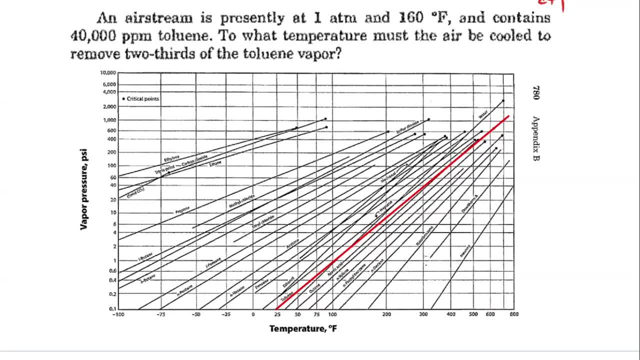 the volatile organic compounds by using this vapor pressure or by using the process that's called the condensation. Right, so what we do is we just lower the temperature, because if the temperature is lower, then the vapor pressure also gets lower. What that means is the 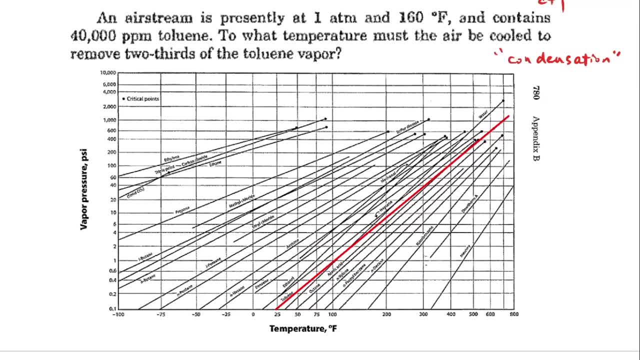 what that means is the partial pressure of this vapor might be above the vapor pressure at a lower temperature. Right, in this way, the extra vapor pressure or extra vapor are going to condense and form liquid and then get collected. right, So we give the example that we're talking about. 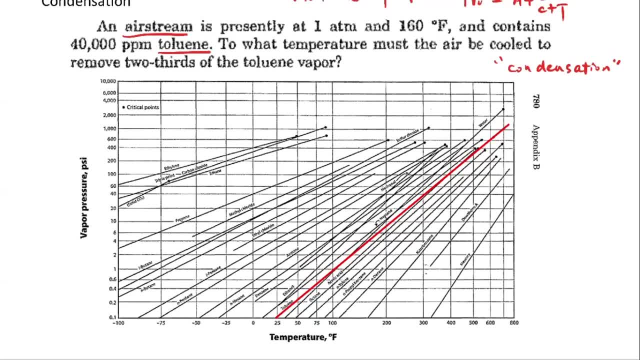 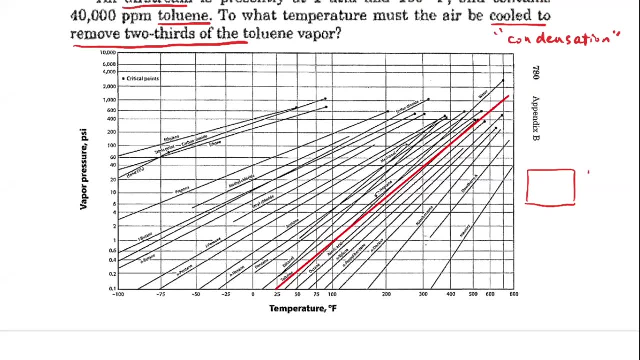 an airstream that has existing toluene inside right And then we wanted to cool it down to remove two thirds of the toluene vapor. So a direct way, or more easier way to think about this picture is, let's say: this is the original state at one atmosphere. 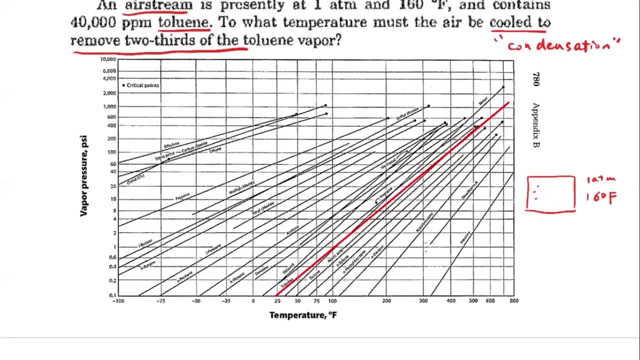 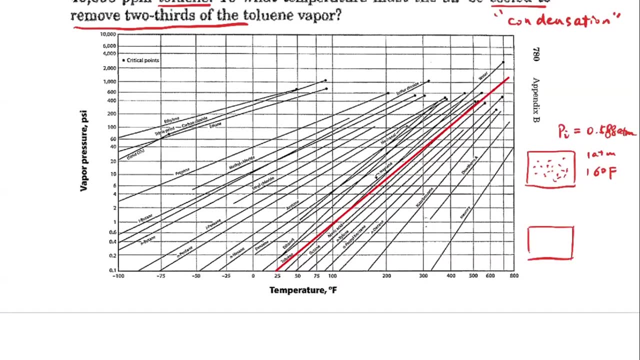 160 Fahrenheit. right, We have quite many vapors here, So it turns out that the partial pressure here is 0.5858 atmosphere. Okay, so what we want, finally, is we cool it down. By cooling it down, we're going to have less vapors inside. 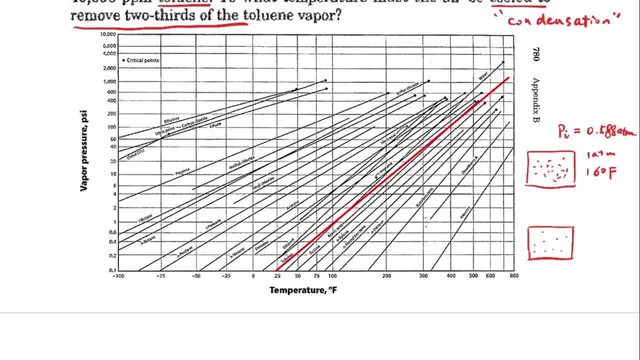 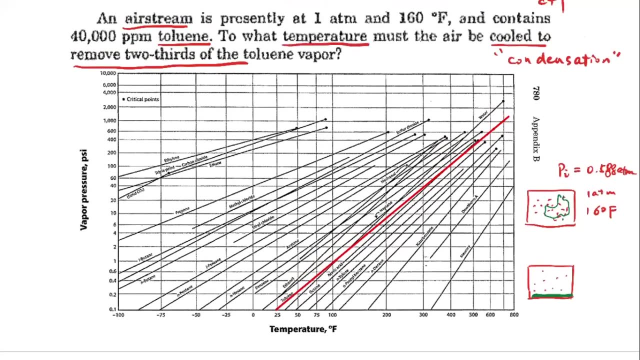 And this is because many of these existing vapor molecules actually get condensed into the liquid right, Just get collected at the bottom of the duct here, okay, So what we're trying to do is we're trying to find the temperature that can give the vapor pressure. 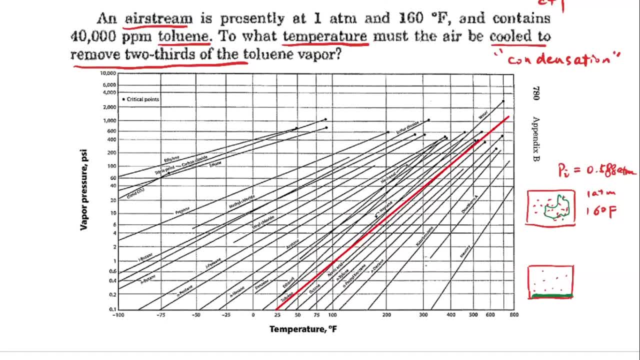 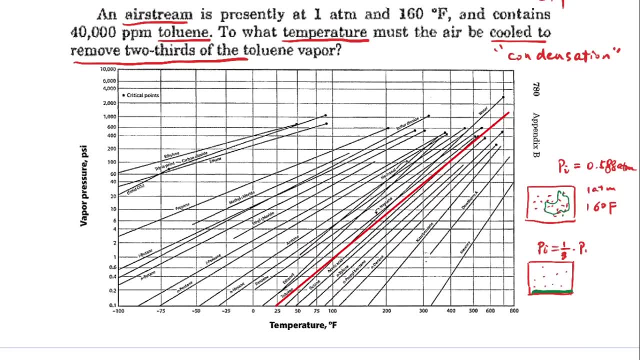 that is, one third of the original vapor pressure. Okay, so we can calculate that by taking a third of the original vapor pressure, That turned out to be 0.196 atmosphere. right, And what this means is that once we cool the temperature down, 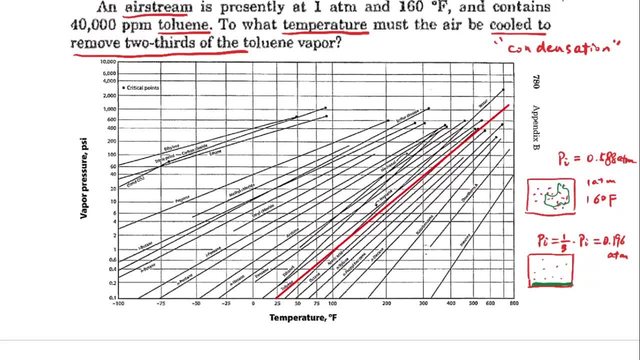 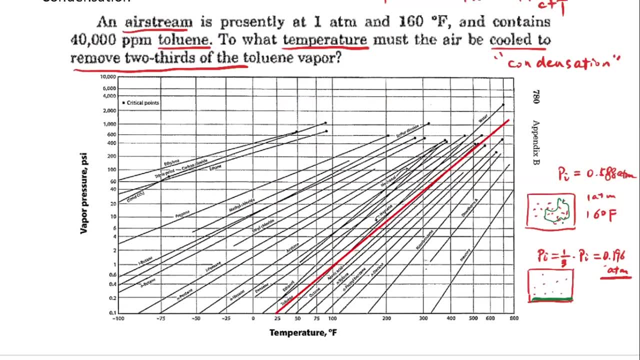 the vapor pressure is always going to be equal to the partial pressure, So it's always going to follow this straight line here. And then we just need to look at this point, which has around 0.2 atmosphere, or 0.2 atmosphere. 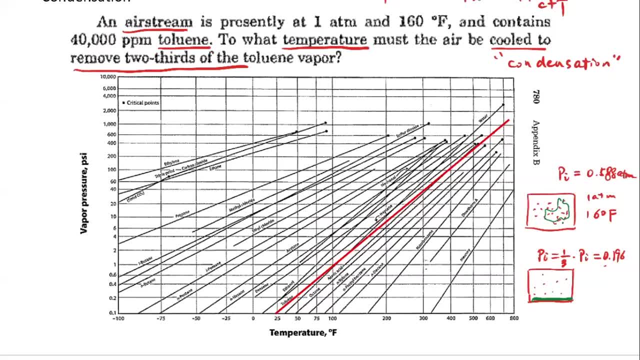 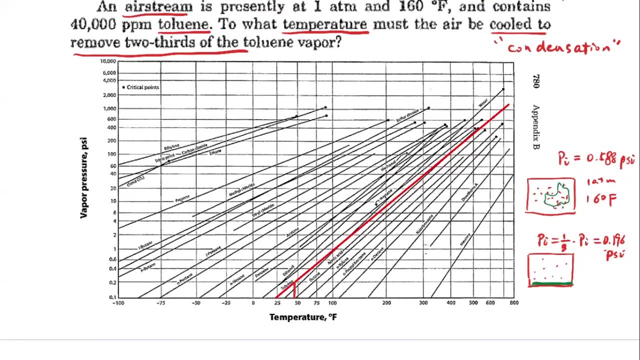 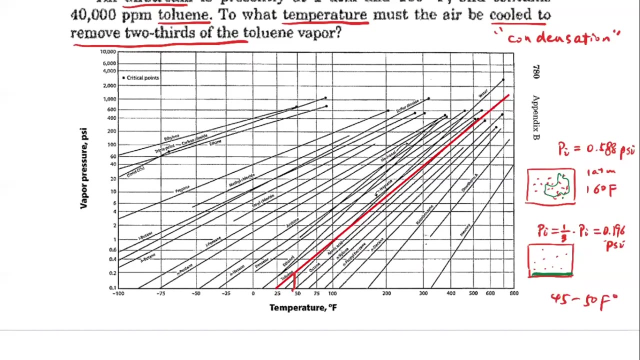 It's PSI- okay, around 0.2 PSI, And you can locate that point, which is around here, okay. So, therefore, you can find the temperature, which is around 45 to 50 Fahrenheit. Okay, so this is how we can use the condensation. 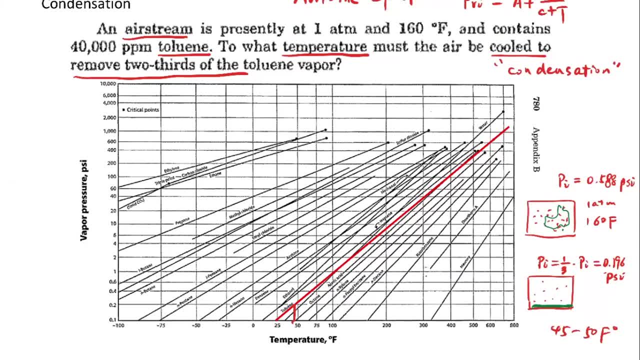 to remove the VOC from a gas stream, And we also mentioned that this is a passive method because the temperature of the flue gas is always cooling before we emit it to the atmosphere, right, So it's naturally happening. But then we may have the question: 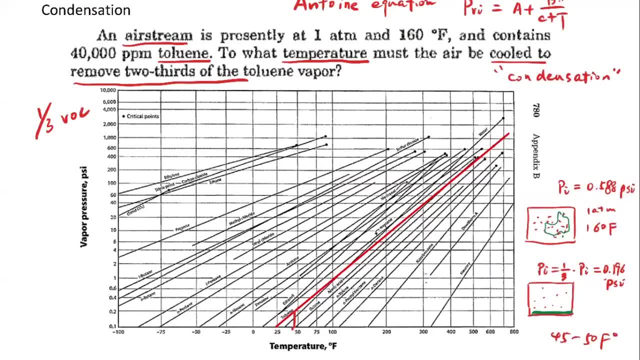 what about the remaining one third of the VOC? So we have to use some passive method, We have to use some active method to remove these VOCs And this class. we're going to have an overview of all of the methods we can use to remove the actual VOC. 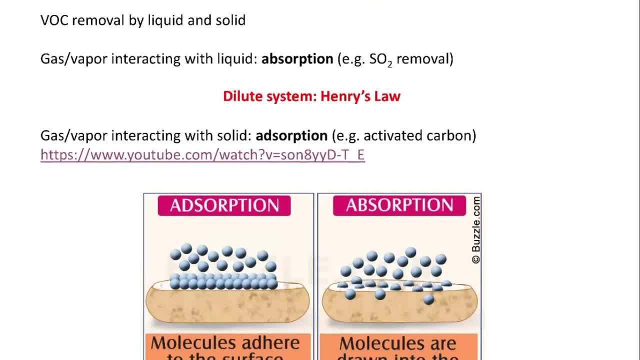 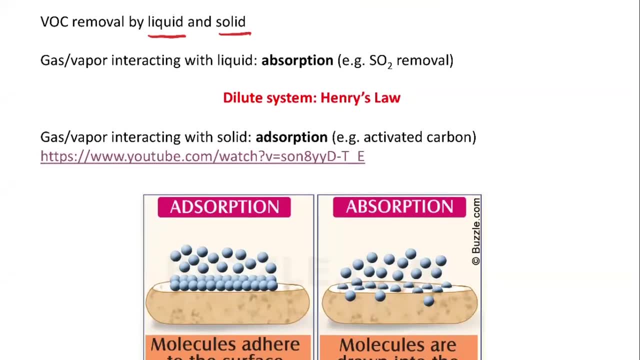 Okay, so the VOCs can actually get removed by liquid and solid. okay, So for different processes, let's say the VOC removal by liquid, it's generally called the absorption, And for the VOC removing by removed by the solid, this process is called adsorption. okay, 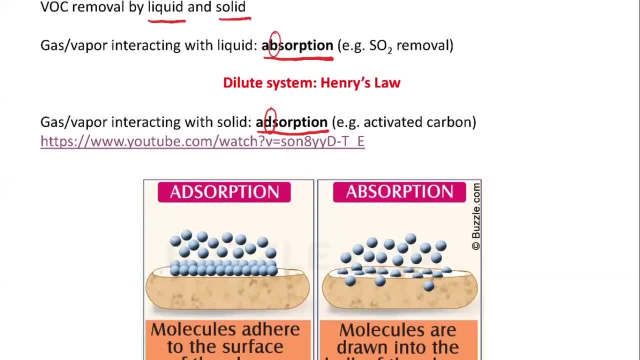 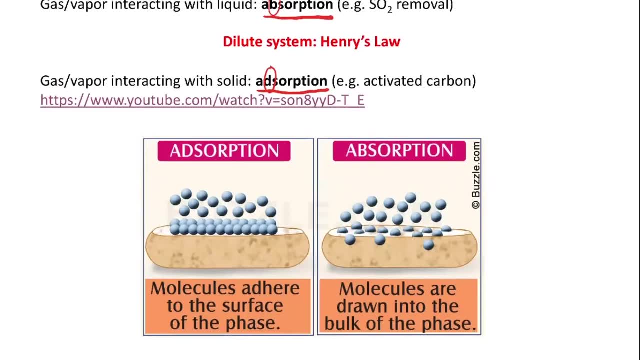 So there is some difference here, right? So absorption generally means that let's say, these are the VOC molecules. okay, So these molecules can penetrate through the liquid, right? Well, this means that the molecules are drawn into the bulk of the phase. 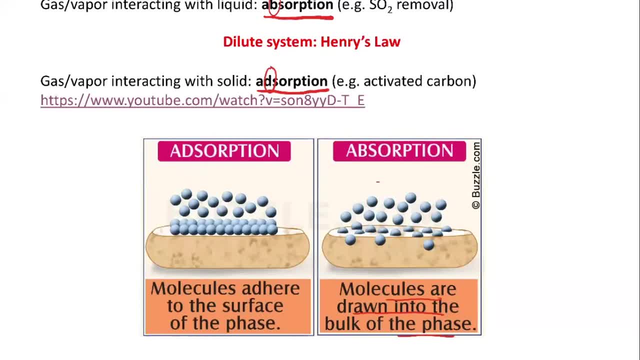 So basically, not only the VOCs are existing outside. once they get in contact with this medium, let's say the liquid. here they can get attached to the surface, but they can also penetrate inside the liquid. okay, So you can think of this process as: 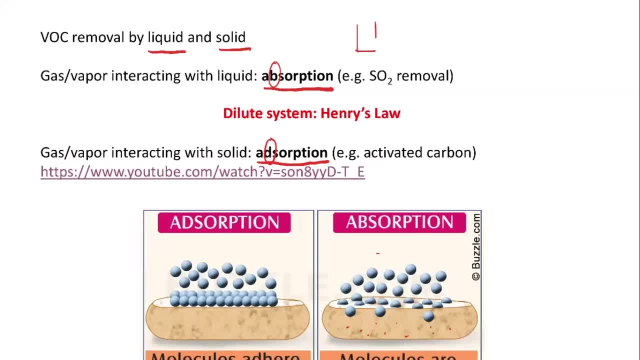 let's say we have a cup of water here, Okay, And then we have carbon dioxide and we're trying to make soda, right. So what soda means is that these carbon dioxide molecules are not only existing at the surface, they're existing everywhere in this liquid. 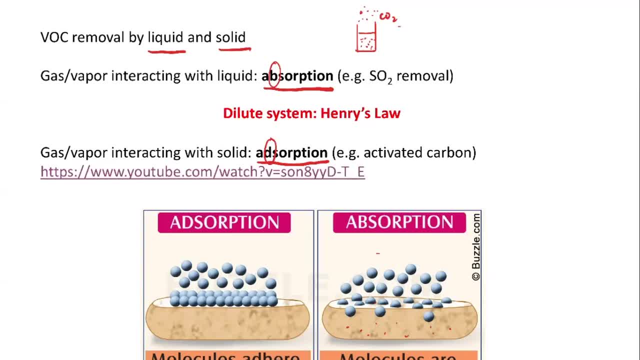 So basically, we can say that the carbon dioxide are absorbed into the bulk of the liquid. So this is indeed the case, because whenever you shake the soda bottle, say Coca-Cola, right, You can see the water, you can see the gas coming from everywhere from the liquid. 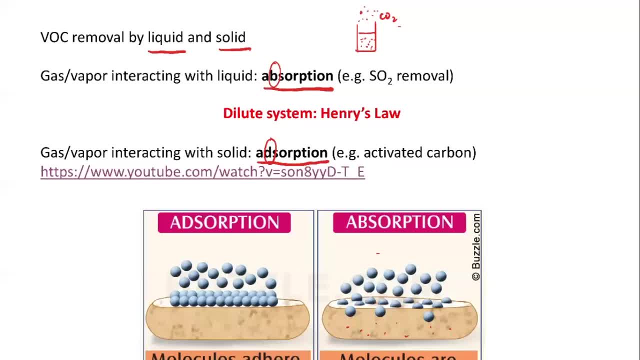 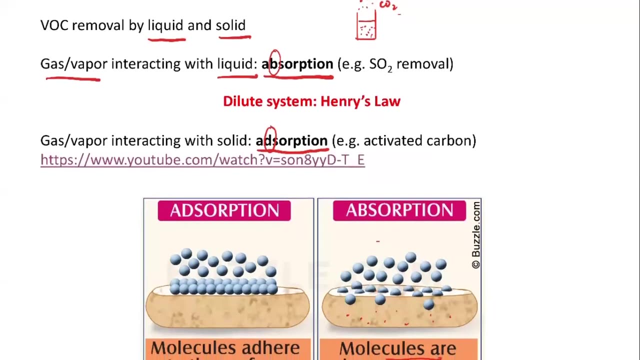 It's not only happening at the surface of the liquid. So the interaction between the VOC or the gas vapor with the liquid, if it's penetrating inside the liquid, we call that absorption, okay, And if we talk about these gas interaction with a solid. 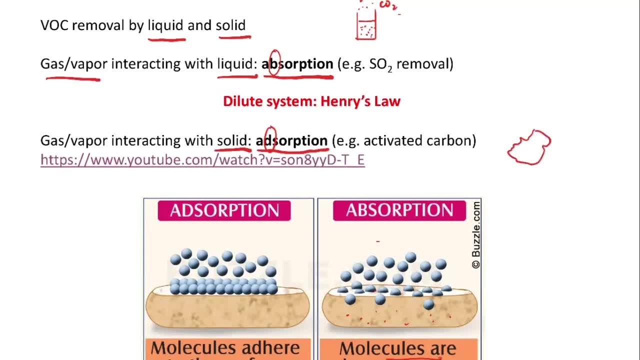 one thing we know for sure is that if we talk about the solid particle, let's say sandstone or something else, right? So the gas molecules, when they're interacting with solid, they're not going to penetrate inside, They're only going to get attached at the surface. okay, 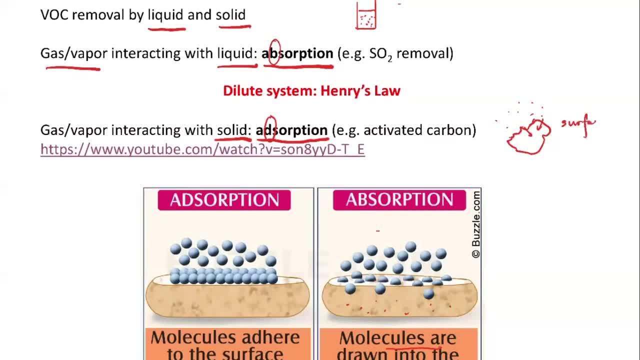 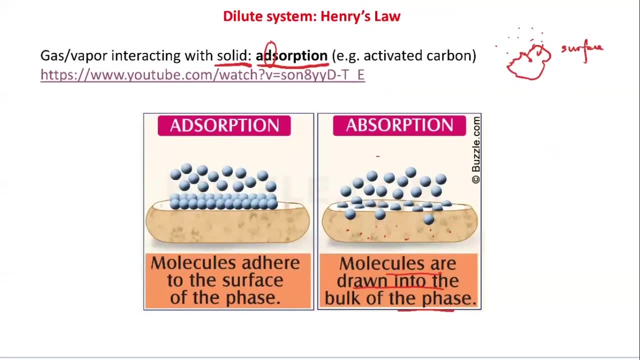 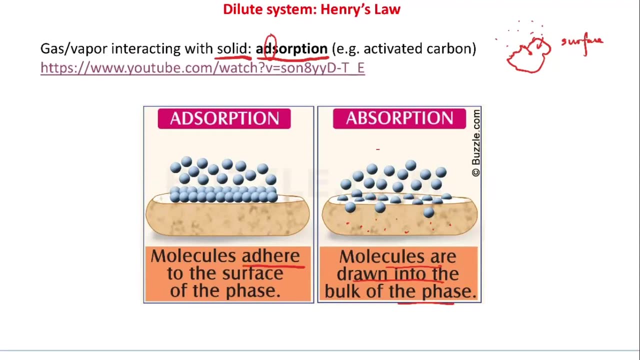 So this process that's happening at the surface of these solids is called adsorption. So I think you can show, you can see that more clearly from this picture here. So basically these molecules are just at here to the surface of the face. 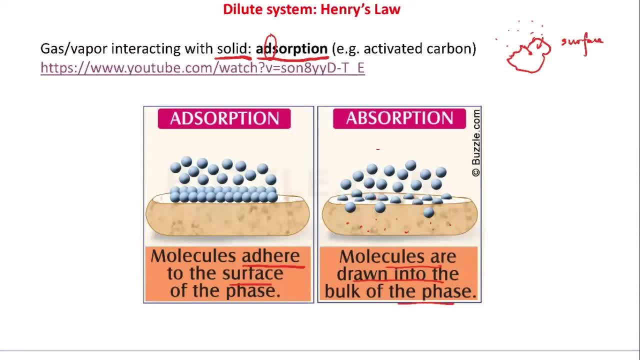 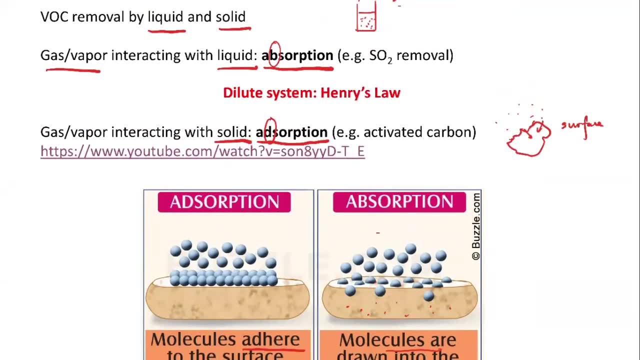 They're not penetrating inside this solid here, And this is called adsorption. okay, So we can go through this adsorption, which is the gas liquid interaction, first, And to determine how effective these liquid can remove the VOC, we should use the Henry's law. 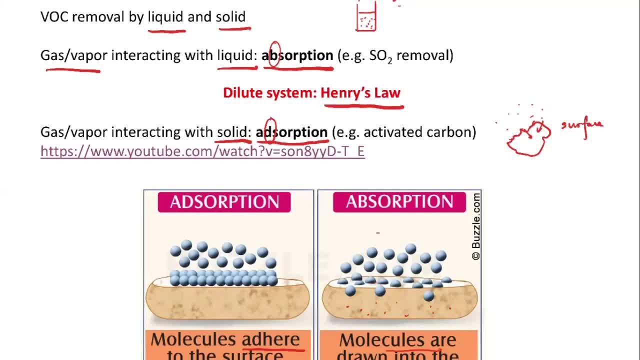 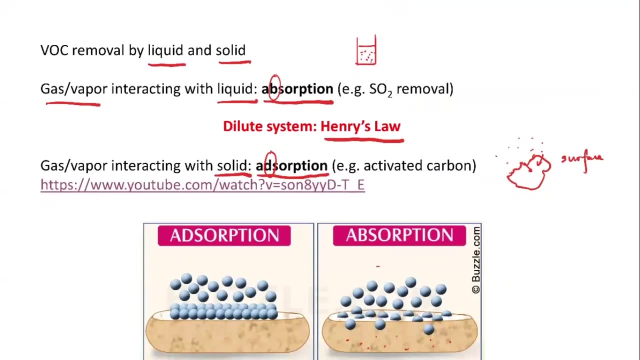 to determine how effective this process is. So basically, the Henry's law determines the partial pressure. Let's say we still use this bottle or cup as an example. okay, So it basically determines what is the vapor pressure of these VOC at the surface of the liquid. 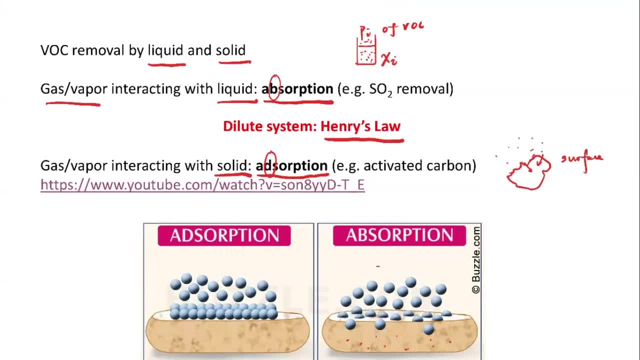 and also, what is the mole fraction of this VOC that's in the liquid? okay, So what Henry's law means is that this vapor pressure, or the partial pressure of this vapor at the surface of liquid is going to linearly increase with the mole fraction of these VOC that's in the liquid. 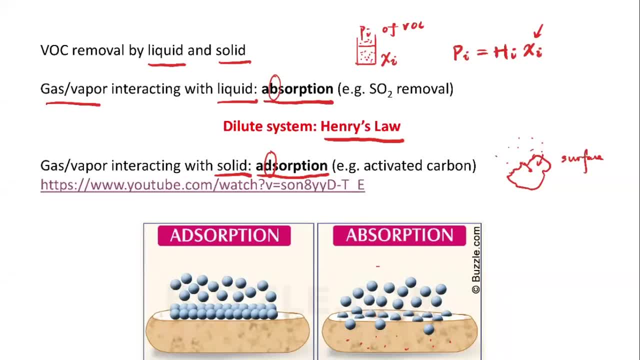 Okay, so if I label these out, the XI is called the mole fraction, So basically it's just the number of the VOCs divided by the total number that's in the liquid. okay, And then the PI here is the partial pressure. 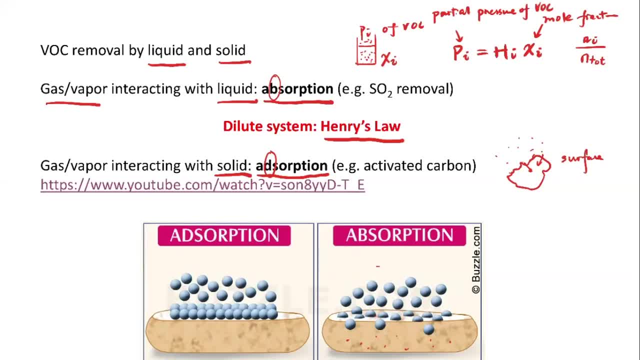 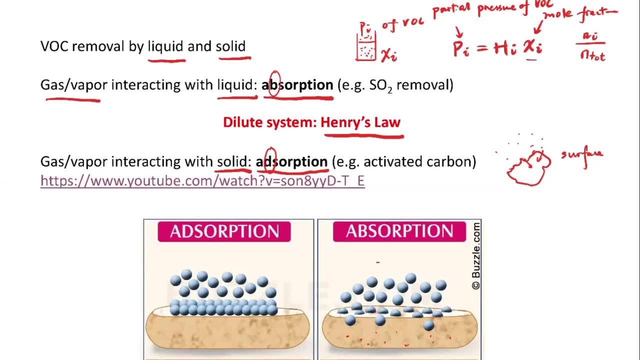 of the VOC. okay, So what this means is that if we increase the mole fraction of this VOC, then the partial pressure will also increase. So you can think of this process as, let's say, we start to pump in some alcohol inside. 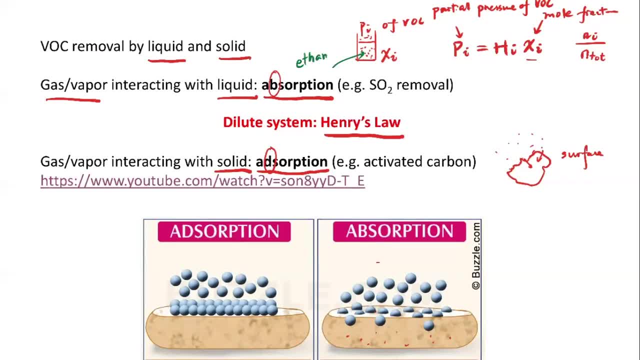 Again here. now we have a very, very high water loss, right? Let's say ethanol, Okay, so we know that for water, if we zoom it in, okay, Change it to a larger cup here. So originally there are a lot of water molecules. 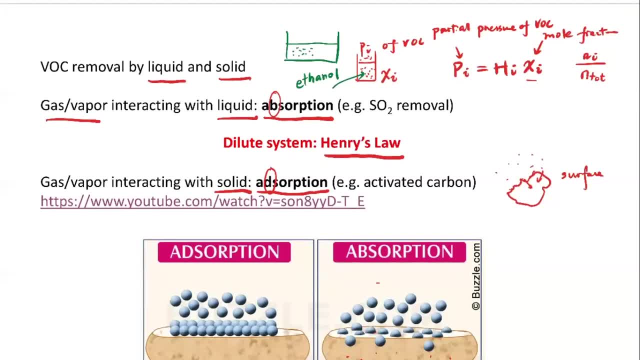 inside the liquid right. We know that the water molecules are going to get evaporated. They're going to establish an equilibrium right. So for water, they're going to establish an equilibrium right. So for water, they're going to establish a equilibrium. 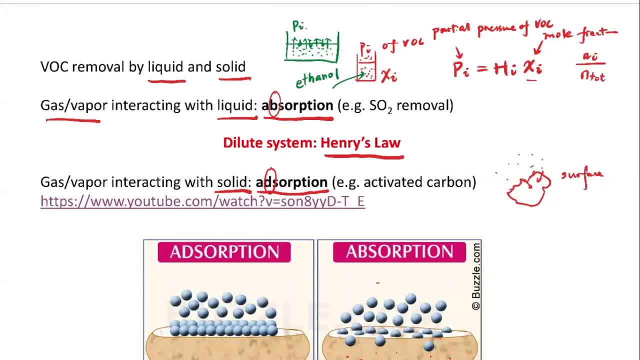 establish a vapor pressure that's above the liquid here and now, if we start to add in ethanol here. so for the ethanol ethanol liquid, they're also going going to establish this equilibrium. okay, so if basically this um current law, what they tell us is that the vapor pressure that's 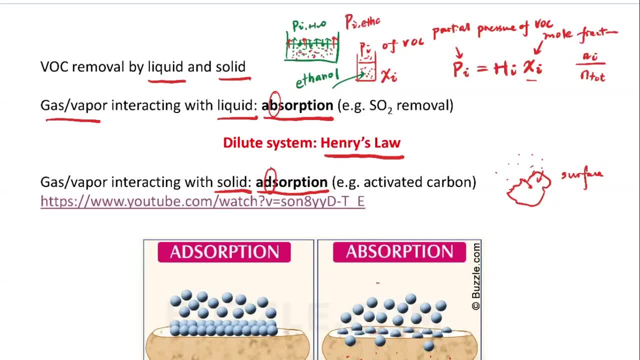 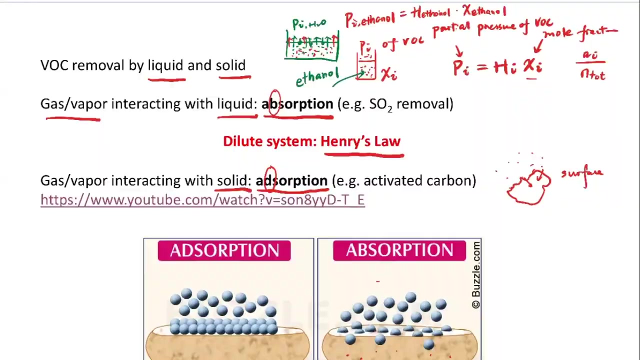 established by the alcohol is going to be linearly increased, going to linearly increase with the, with the mole fraction of the alcohol inside. okay, the more alcohol you have, the higher the vapor pressure, the higher the partial pressure there will be. okay, so we can, um, basically show an. 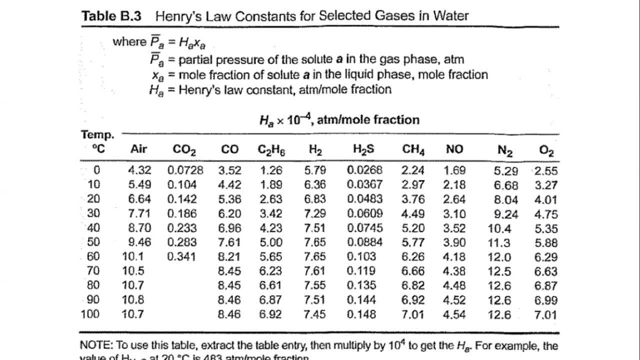 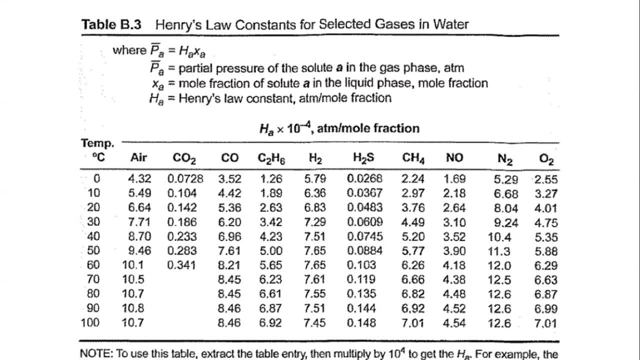 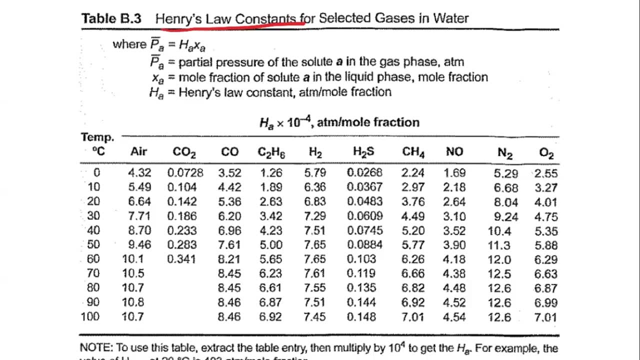 example here, um, so this is a table that's shown on the back of your textbook. this is a basically in the appendix that's showing the list of this henry's loss constant. okay, so you can see that henry's law basically determines what is the partial pressure above the liquid for a voc species that has 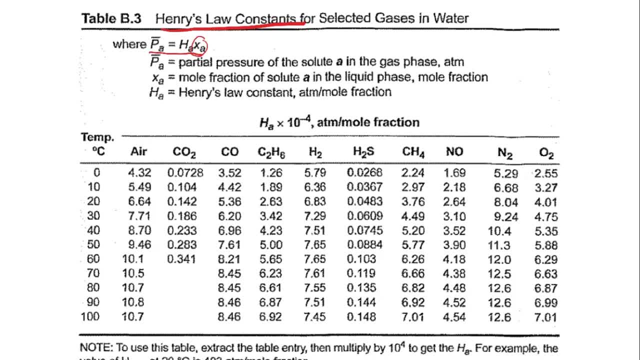 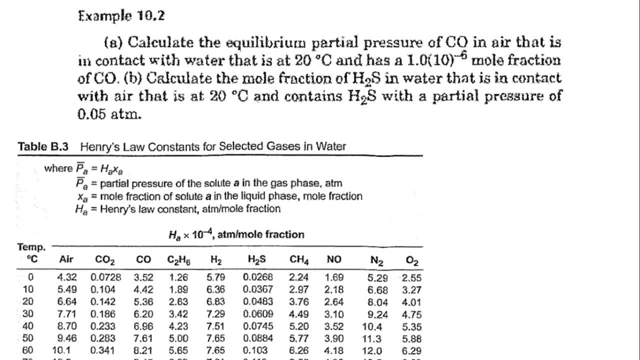 certain mole fraction inside the liquid. okay, and we're showing the list of the henry's loss constant that's showing here. so, for example, if we're trying to do some calculations, all right. so this problem, i want us to calculate the equilibrium partial pressure of the carbon monoxide in air that is in contact with water and at 20 celsius. and then we also know: 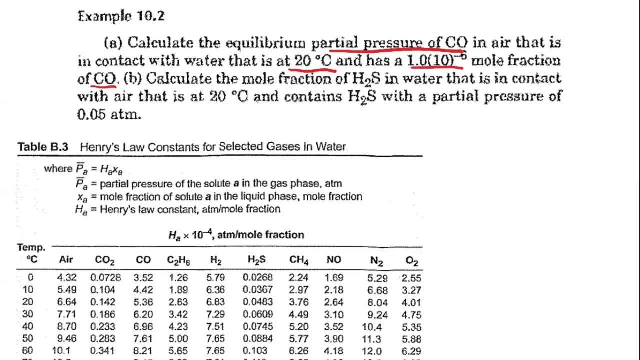 that the mole fraction of the carbon monoxide in the liquid is 1 multiplied by 10 to the negative 6.. okay, so what this means is that if we talk about this cup of water again, we have just a few carbon monoxide molecules in the liquid. okay, and then their mole fraction, basically. 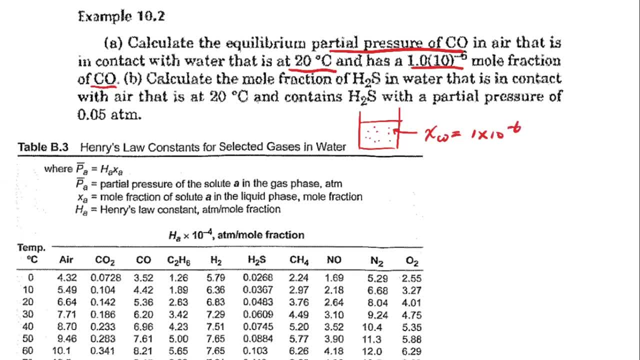 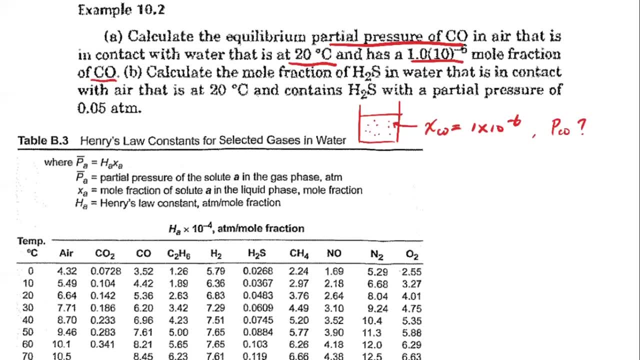 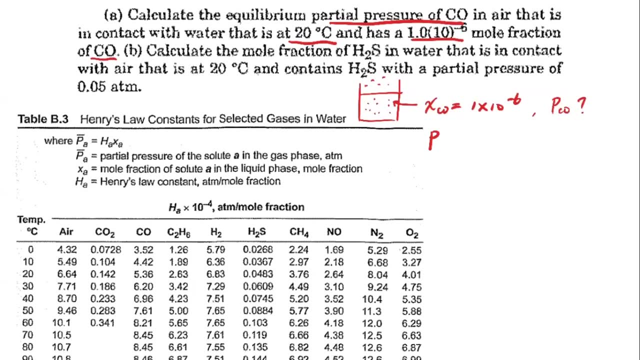 is 1 multiplied by 10 to the negative 6. okay, and it's asking us for what is the partial pressure of the carbon monoxide that's at the top of this liquid? here, so we can directly use the um henry's law. right, we have pco equal to. 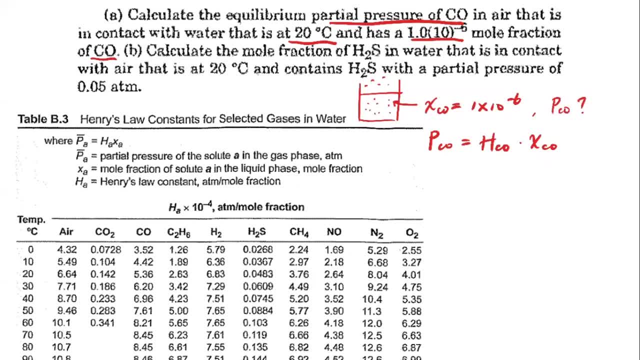 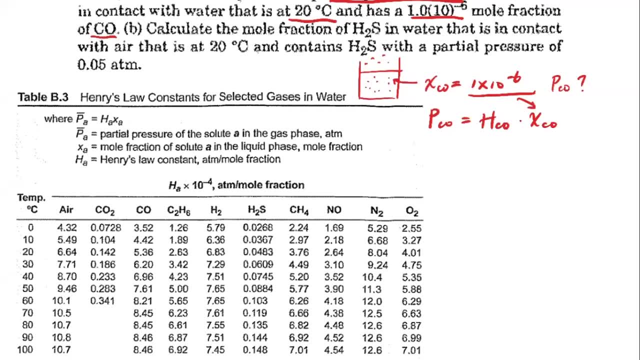 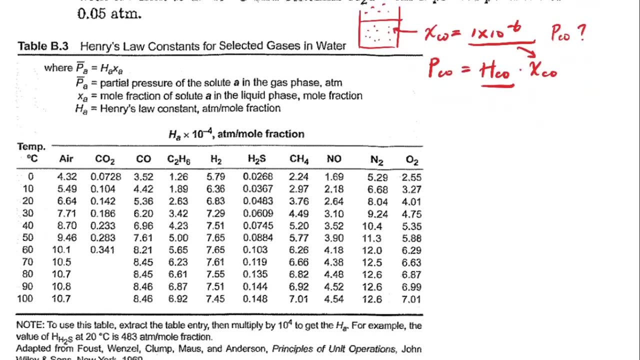 hco multiplied by xco. right, and we can directly plug in this value here. this is the mole fraction of the carbon monoxide in the liquid. we just need to find out what is the henry's constant so we can refer to this table here and zoom in a little bit. basically looks a. 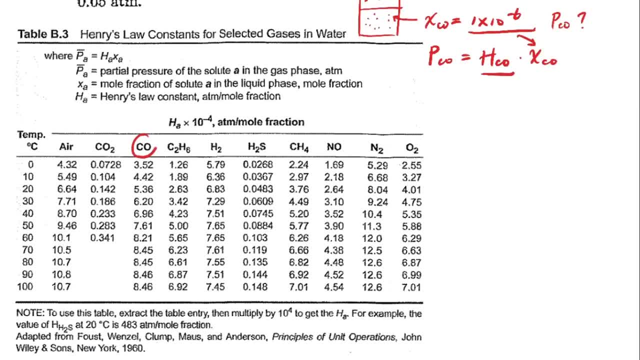 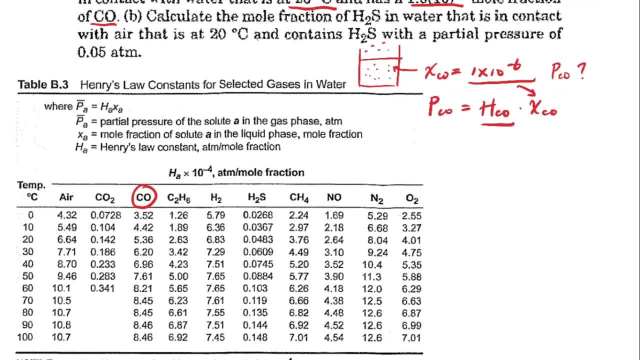 little bit smaller here, but we can still find out co is in this column here. and we should also notice that the henry's constant is dependent on the temperature of the system. okay, and generally, the higher the temperature, the higher the henry's constant. you can see lower temperatures, we're. 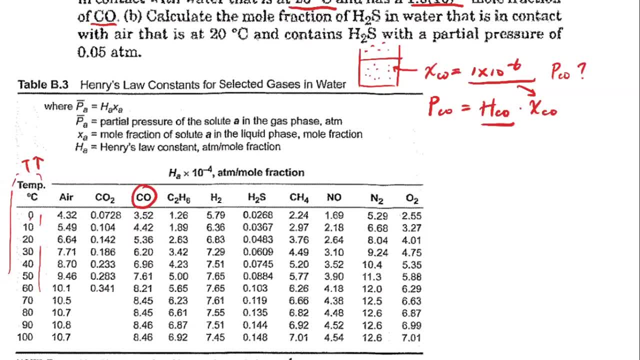 going to have lower value. so basically it means that it means that if you have a boiling water means that you can basically pump in more vocs inside the water, since inside a higher temperature and absorb more VOCs. But right now, if we just look at the carbon dioxide, 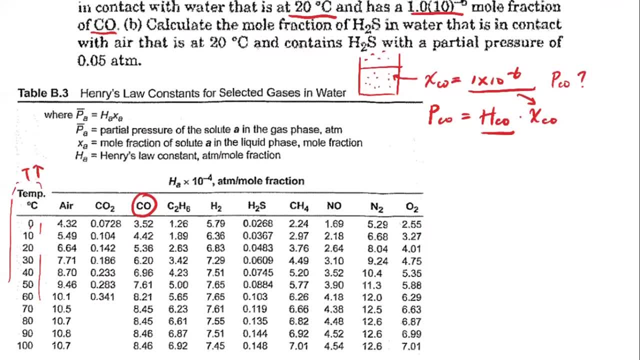 and then if we find the value- here we're talking about 20 Celsius, that is here right- And then we can find the Henry's loss constant, which turns out to be 5.36.. But we also need to notice that for this table. 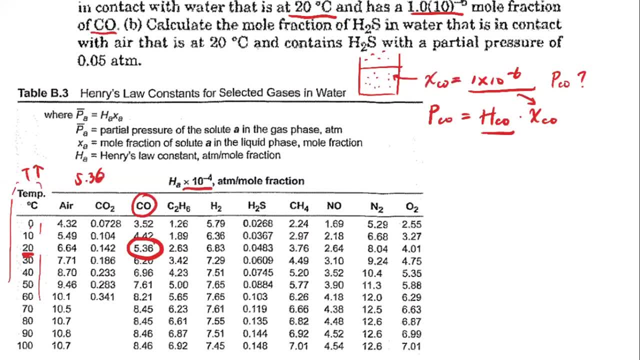 it's showing the values by multiplying 10 to the negative 4 to the Henry's constant. So what this means is that the Henry's constant for carbon dioxide at this temperature is going to be 5.36 multiplied by 10 to the fourth. 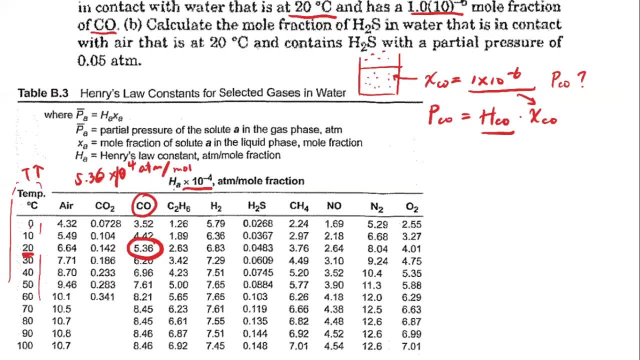 of atmosphere per mole fraction. Okay, so this is how we can find the Henry's constant. So first we find this value here and then we multiply that by 10 to the fourth. Okay, so since we have this value here, we can plug it in. 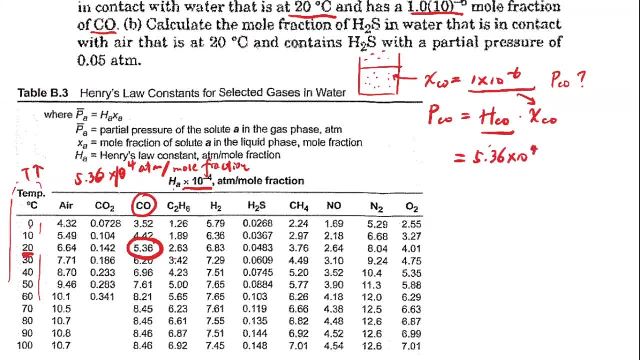 That's 5.36 multiplied by 10 to the fourth, And then we multiply that by 10 to the negative six. Okay, so that turns out to be 5.36 multiplied by 10 to the negative two, which means it's 0.0536 atmosphere. 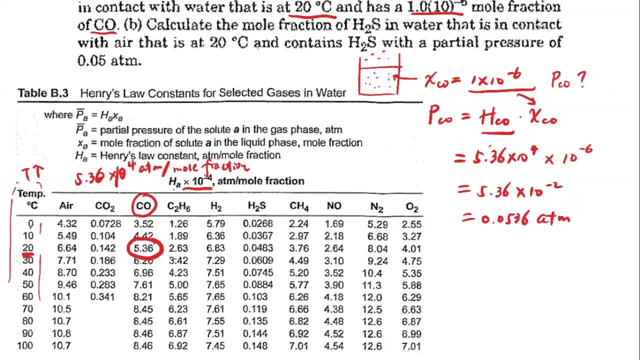 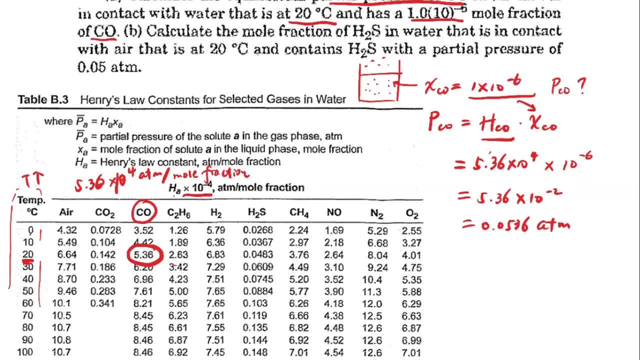 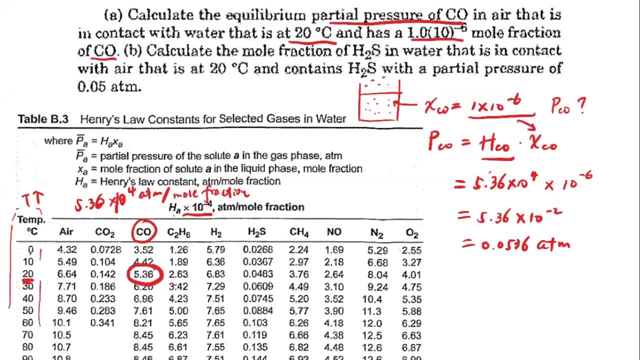 Okay, so it's around 5% of the atmosphere pressure, right? So this is how we can calculate the vapor pressure of certain species. It doesn't have to be VOC, but for all the gas species, when we have an equilibrium between the air and the liquid, 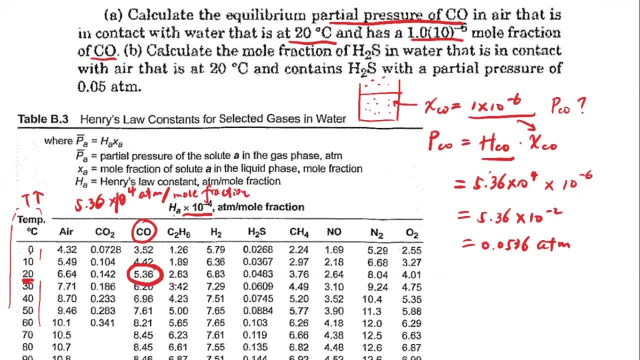 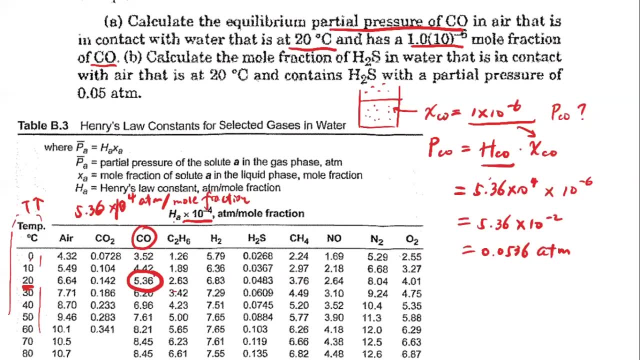 and also the air can get absorbed into the liquid. Okay, so this is the first question of the problem. We look at the second question. So it wants us to calculate the mole fraction of the hydrogen sulfide. Okay, So it wants us to calculate the mole fraction of the hydrogen sulfide. 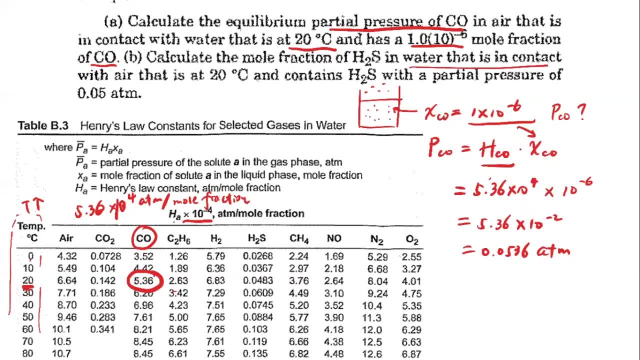 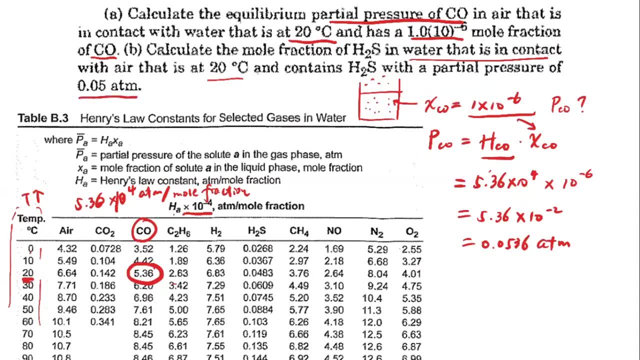 Okay. So it wants us to calculate the mole fraction of the hydrogen sulfide in the water That is in contact with air and at 20 Celsius and contain hydrogen sulfide with a partial pressure: 0.05 atmosphere. So for the second question. 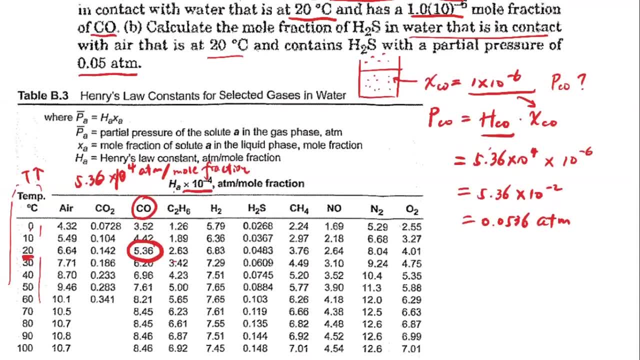 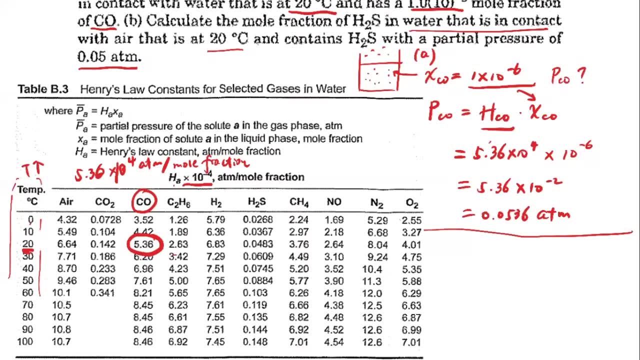 it's talking about how we can calculate the mole fraction if we know the partial pressure at the surface of the liquid. Okay, So if we label this as A, this is B here, So we can still use the Henry's law. We have P, hydrogen sulfide. 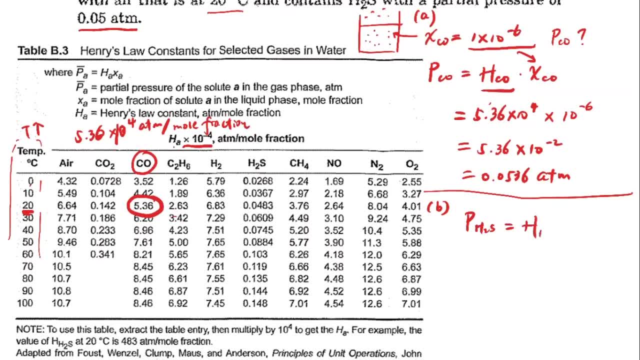 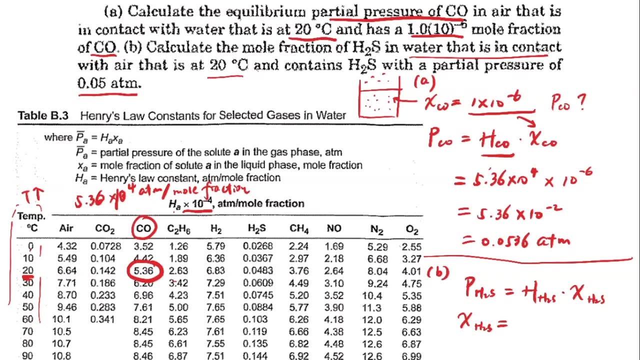 P hydrogen sulfide equal to the Henry's constant of hydrogen sulfide multiplied by the mole fraction of the hydrogen sulfide. So we're trying to calculate what is the mole fraction. So we can rearrange this equation, That is, P? H2S divided by the Henry's constant of H2S. 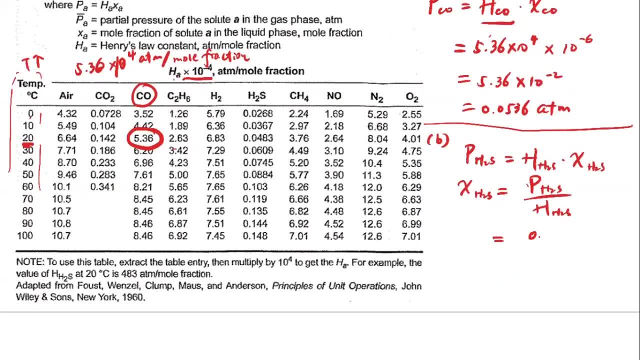 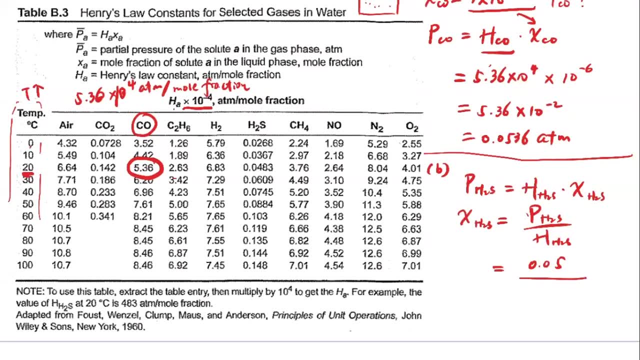 So we know that the partial pressure is 0.05.. We can directly plug it in, And then we just need to plug in the Henry's constant of the hydrogen sulfide. If we go to this table again, you can find that it's this value here, right? 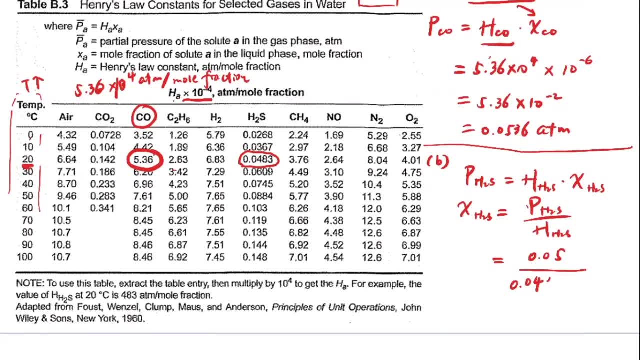 And then we plug in the value of 0.0483 multiplied by 10 to the fourth And then we can calculate what is the mole fraction. So that turns out to be 1.04 multiplied by 10 to the negative four. 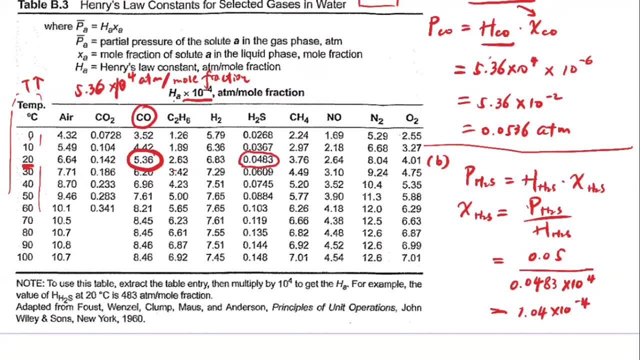 Okay, so this is how we can use this Henry's law to calculate either the partial pressure or the mole fraction of these gas species in the liquid. So this has applications in the absorption of VOCs or other gas species. So we can think of a scenario. 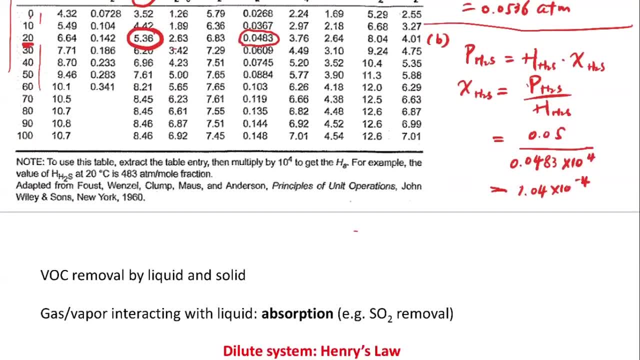 Let's say we have a stream of flue gas, right, And then they're going this way. So what we can do is we can spray water droplets. So it's similar to a scrubber, I would say right. 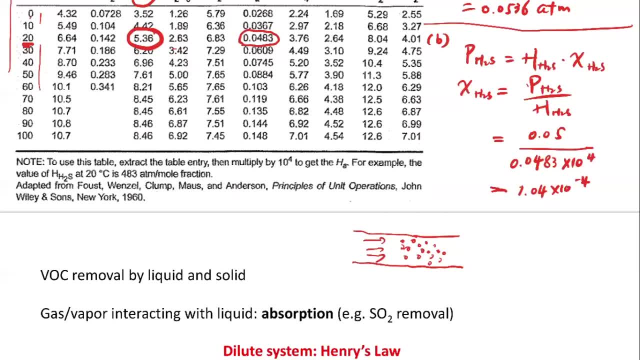 And then we're spraying water droplets And then because of the absorption process, so basically these gas species can get absorbed inside the water liquid. okay, So if we already know what is the partial pressure of these VOCs, right We can calculate. 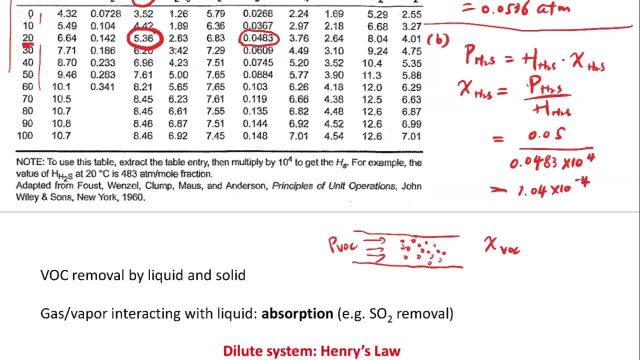 what is the mole fraction of the VOCs in all of these water? okay, I know in this, if we further know what is a quantity and say the volume, total volume of the water, and we can multiply these together and to find out how much of the VOCs are being collected. 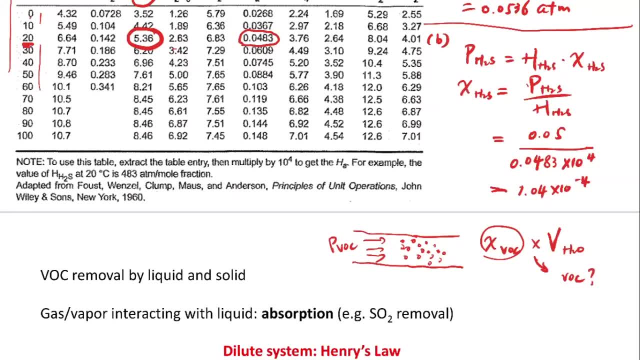 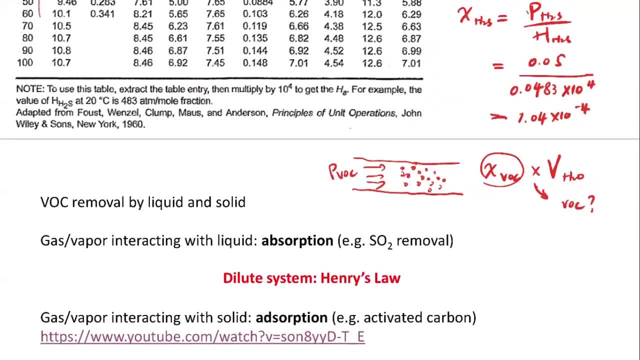 So we can use this absorption process to basically remove the VOCs from the flue gas. okay, And actually, I think, also labeled here, So for the sulfur dioxide removal where we use the limestone scrubber. so the process that's happening is that if we- if you recall the geometry of the scrubber- 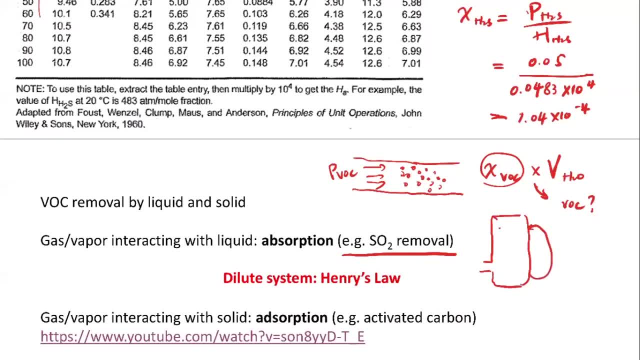 right. we're recirculating the limestone and then spray droplets. that's containing limestone in the droplets- right, and then we're sending the flue gas that contains sulfur dioxide inside, right. so the first process that's happening between the sulfur dioxide and the droplet 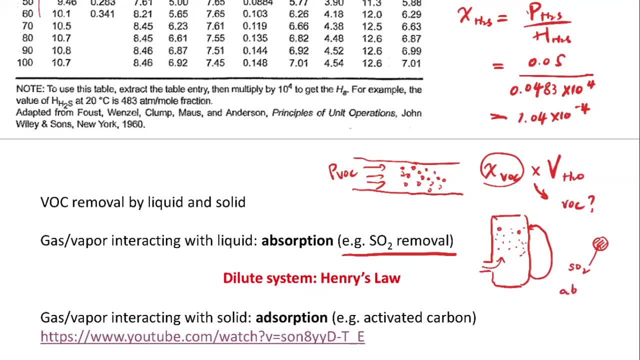 is that the sulfur dioxide have to get absorbed, have to get absorbed into the liquid right, and then the reaction can take place between the sulfur dioxide and calcium carbonate. Okay, so for the scrubber system, it is using the absorption of these gas species in the liquid. 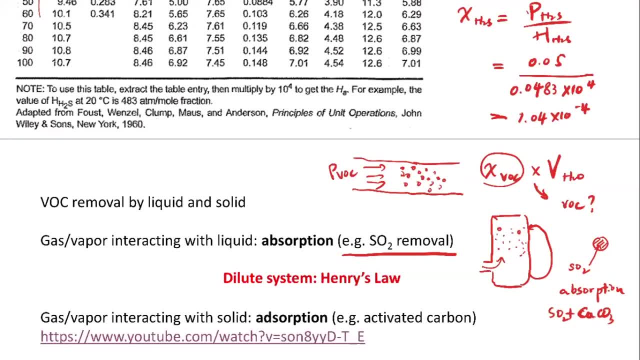 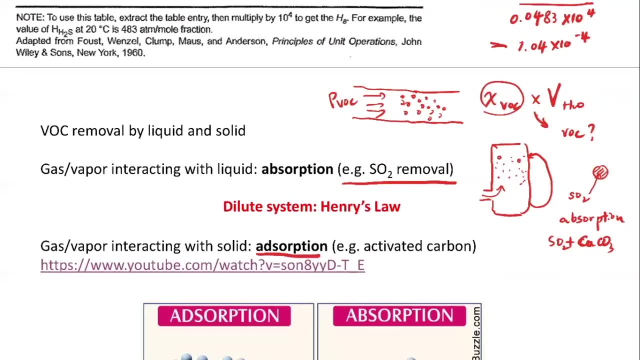 Okay, so that's why we can use this absorption to remove the VOCs, and we can also use the adsorption to deal with the VOCs, and here I actually have a short video which is showing how this mechanism works. So the most commonly used medium for absorbing the 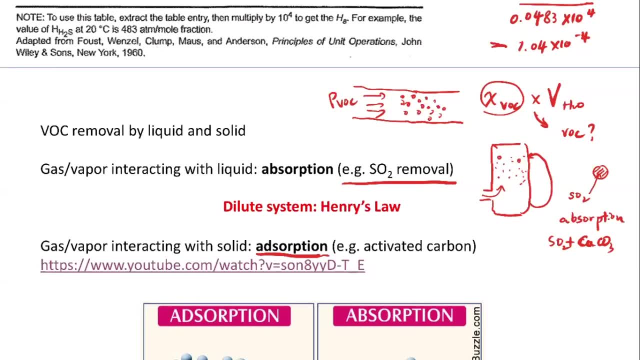 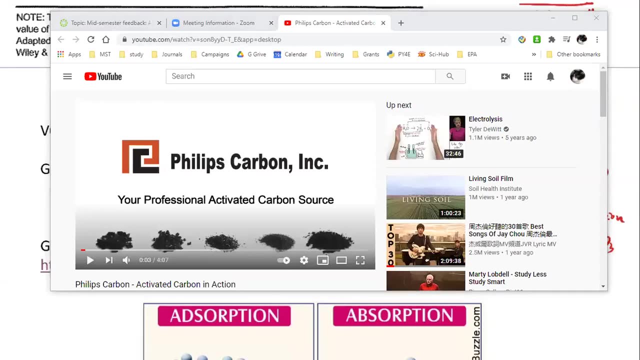 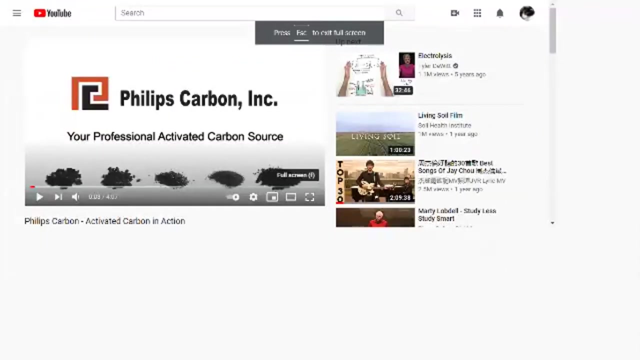 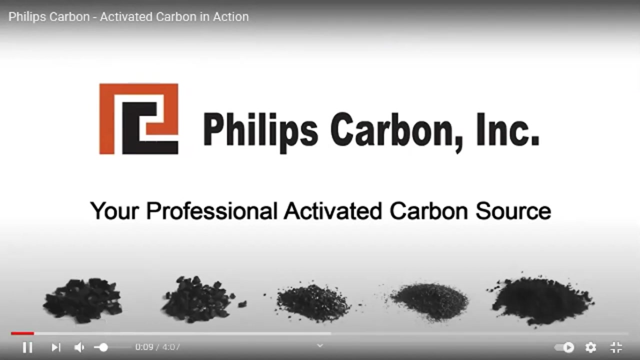 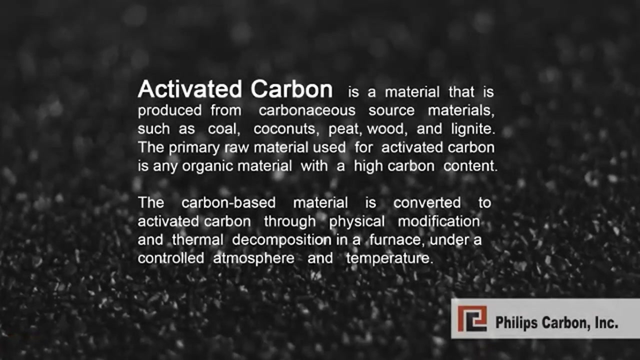 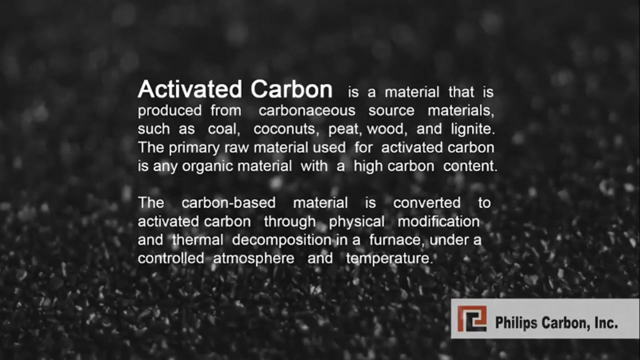 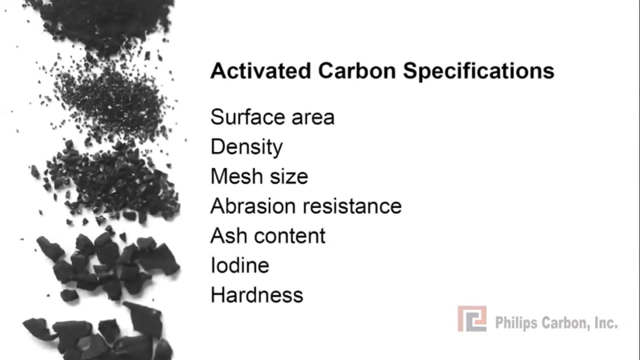 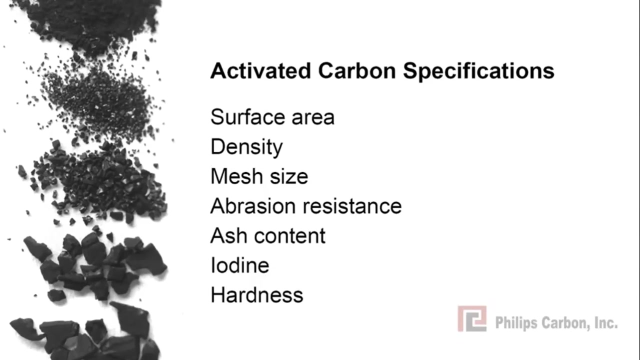 toxic gas species. toxic gas species, not not only VOCs, are the activated carbon. Okay, so this video is going to show you how the activated carbon actually removes these polluted species. Okay, yeah, so the active carbon are basically just mainly made of carbon and be made of. 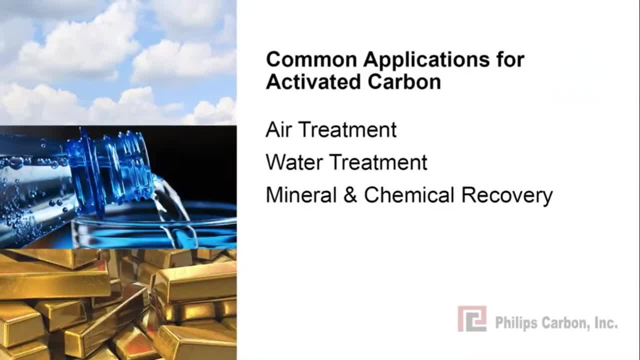 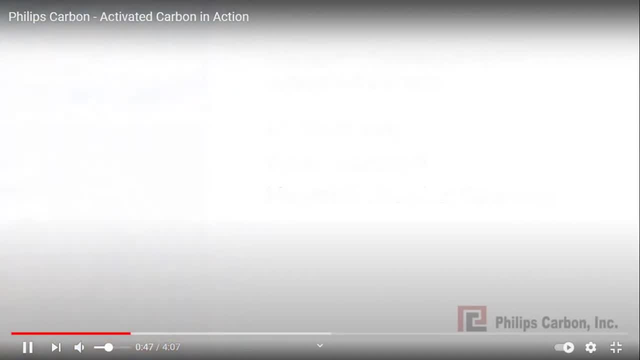 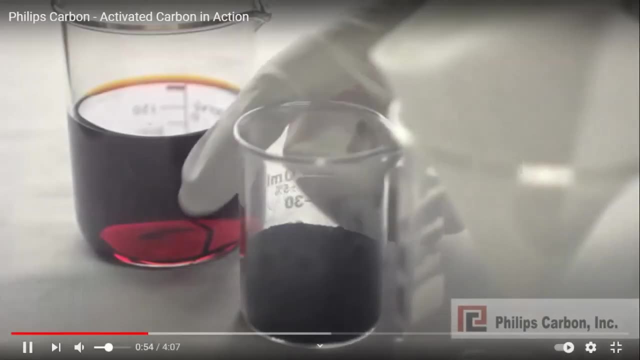 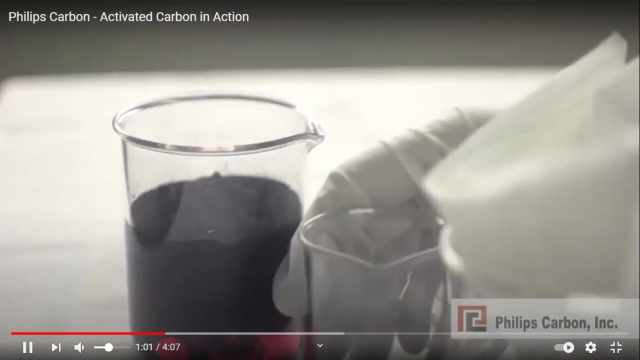 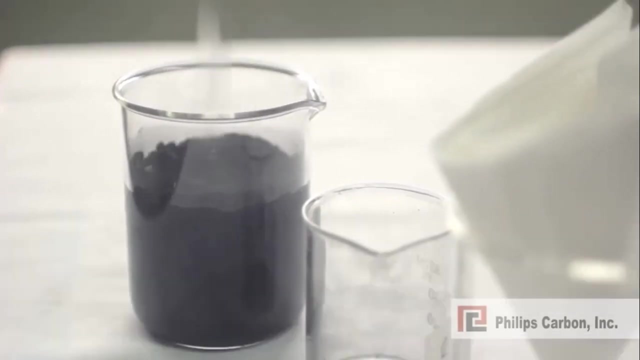 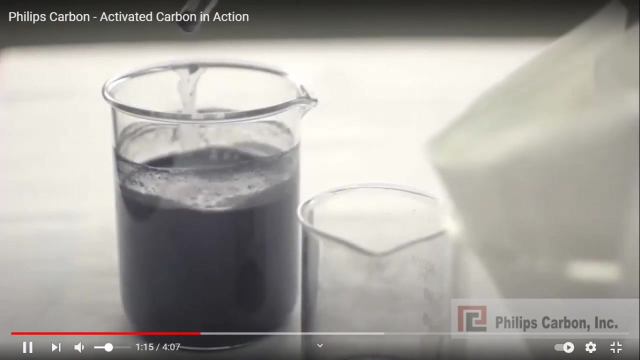 so what this process is showing is that, let's say, have some water that has iodine inside, iron that will get dissolved in the water. theoretically, if we pour the solution through the filter here, it's never going to filter out those ions. but if we add this active activated carbon into the solution, then these iodine are going to. 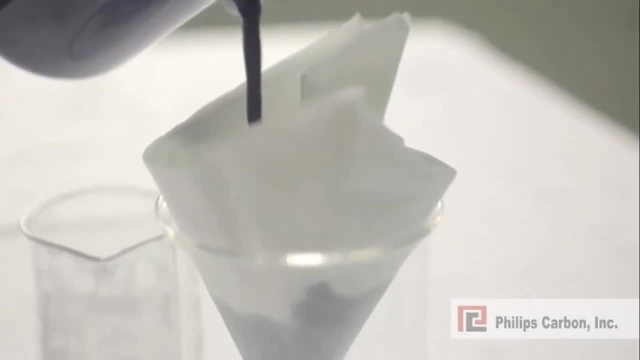 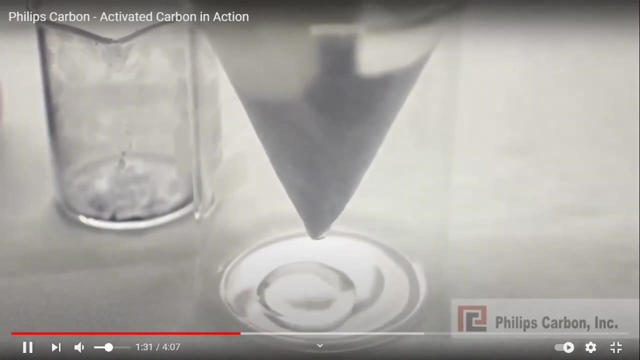 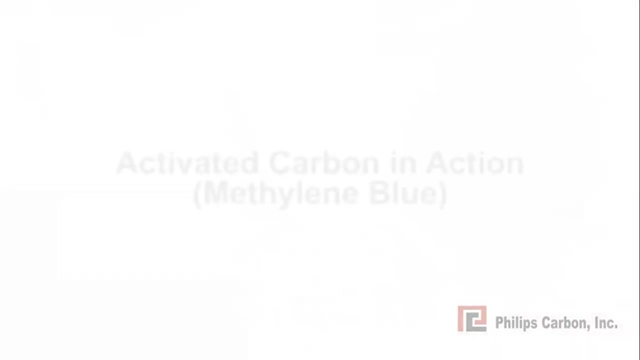 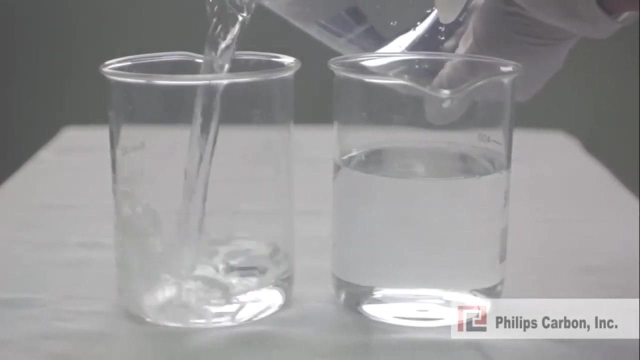 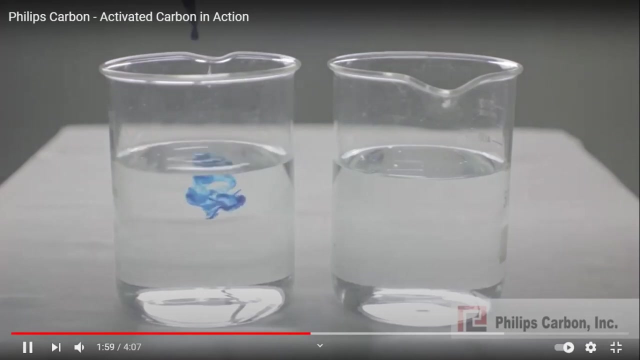 get absorbed on the surface of the activated carbon. now we know that the filter is going to filter out the activated carbon because they're solids and because of that we can get pure water- basically these polluted, contaminated species that get attached to the surface. and what this problem, uh, what this process is showing you is that we add some dyes inside. 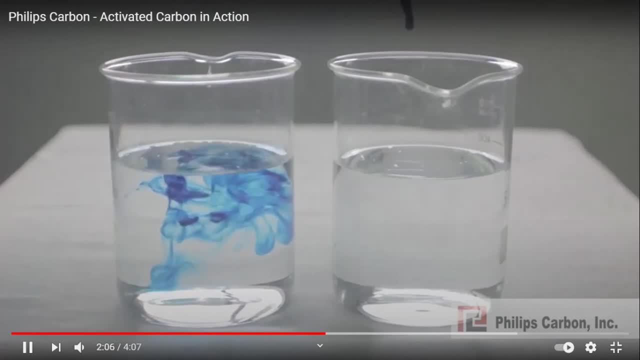 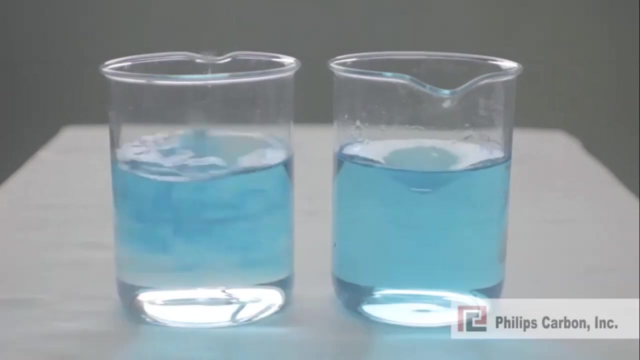 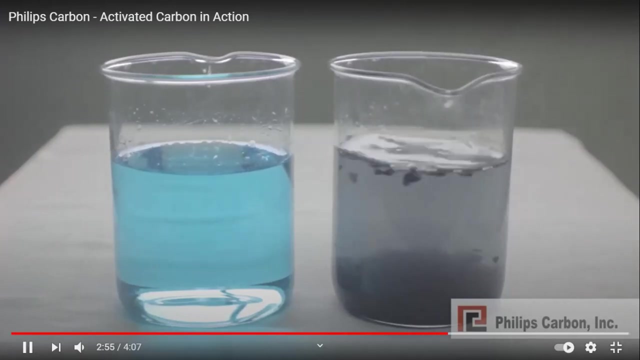 inside the water. basically, the dye is made of organic molecules- almost perfect. it's going to be very difficult by filtration. so now if we add activated carbon inside the solution, we can see that the water is getting purified right because the dye molecules get attached to the surface of the activity carbon. so why the surface is so important? 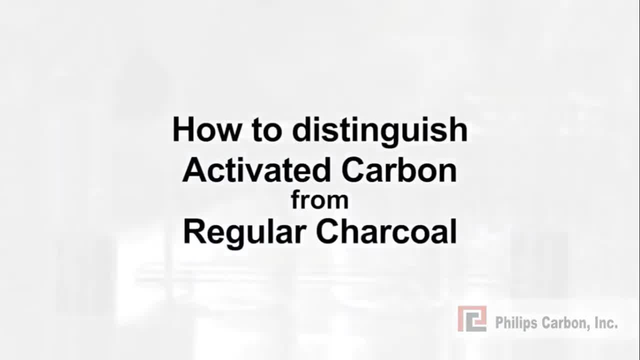 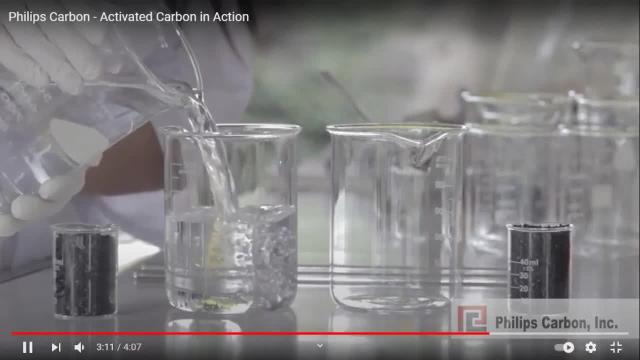 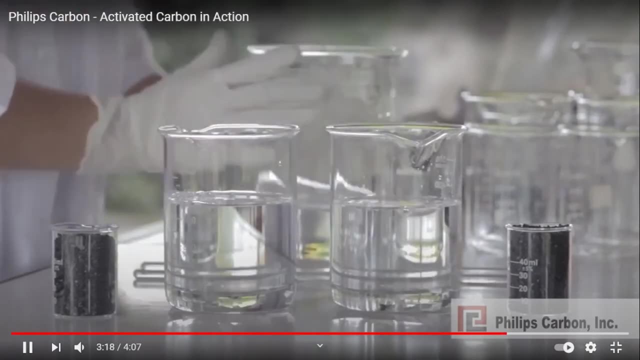 these active carbon have a very surface area. that means it can hold more molecules on the surface of these solids here, and this is telling us what is the difference between the active carbon and typical charcoal. so you can see there are two bottles or beakers of these solids. 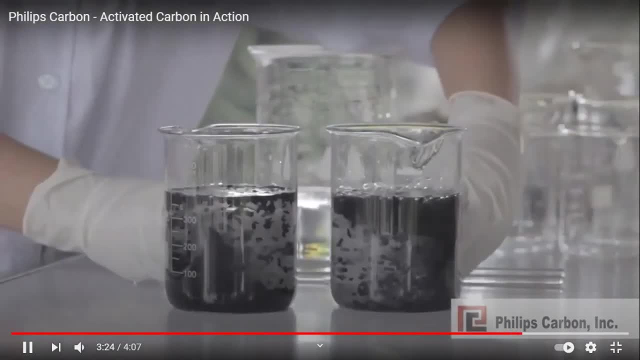 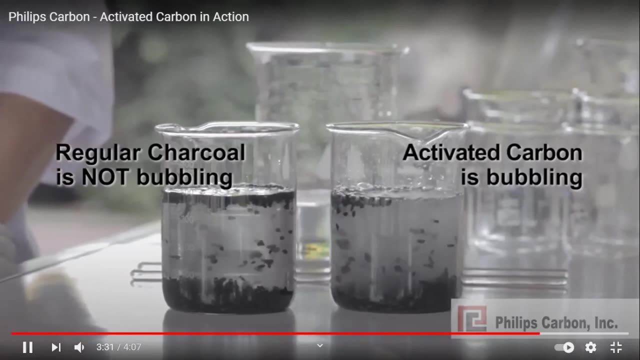 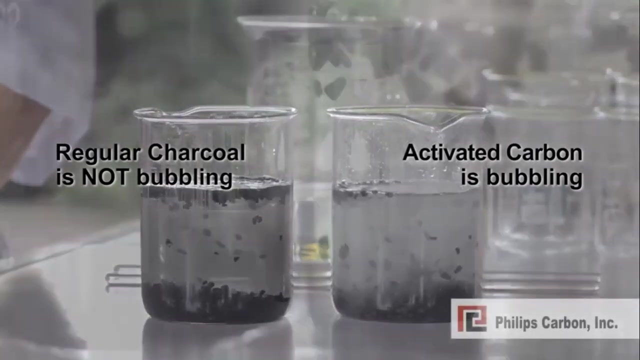 look almost the same by appearance, but if you pour them into the water, see, the regular charcoal is not bubbling, but the active carbon is always bubbling. the reason why it's bubbling is not because of reaction, because these active carbon has a very large surface area, so when you add them in, it brought a lot. 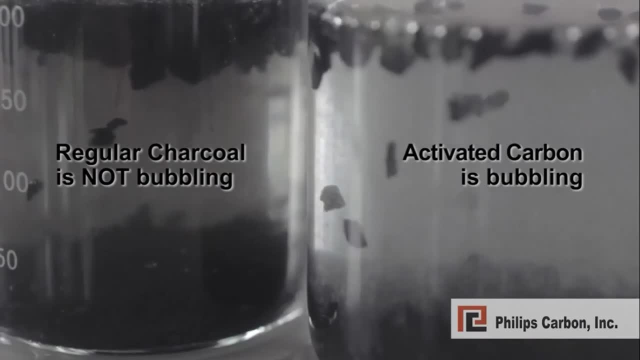 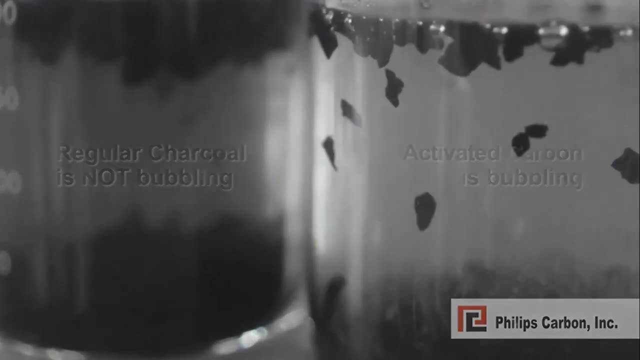 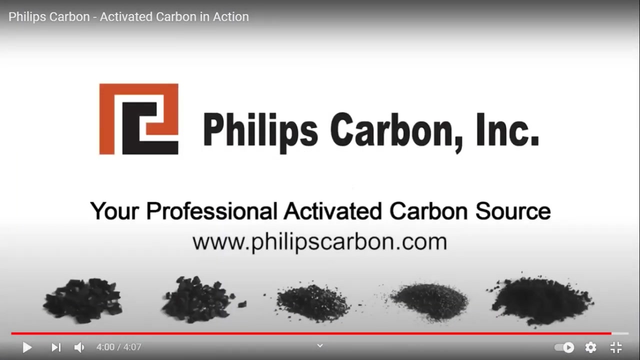 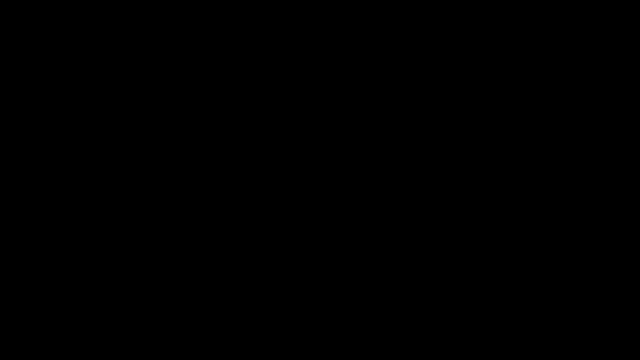 of water. it brought a lot of air molecules inside the liquid. while the water is occupying those surface area of the aggregate carbon, it basically pushes the air outside, right under these water bubbles coming out right. so this is a short video about the activity carbons which come out of the liquid, which is the carbon that we're talking about. 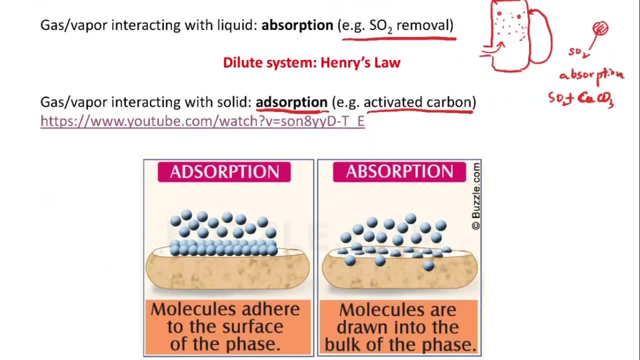 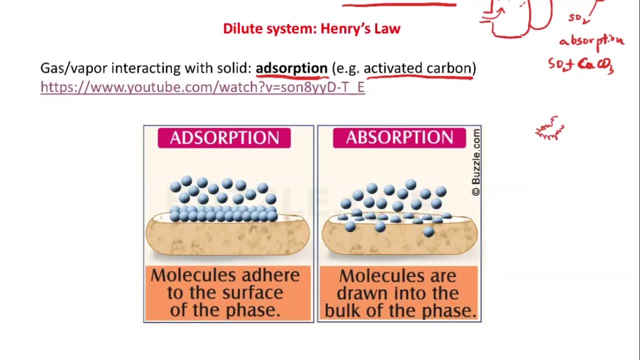 and, as you can see here, these are the preheating ludzie who use these. so let's say, if i draw a schematic of the active carbon, the way they look like is generally has a lot of um, these, um, these extra branches, basically giving them a very large surface area. 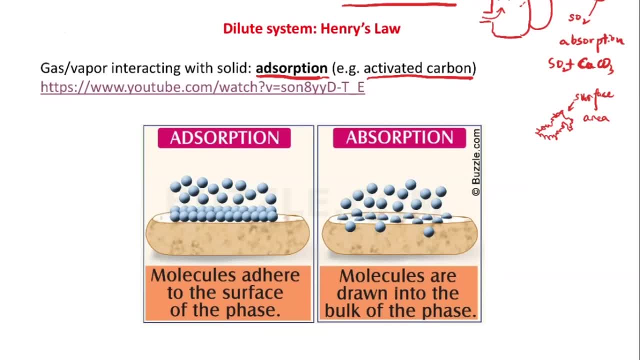 the air bubbles is that if we just put it outside, let's say expose it to the air, then a lot of these oxygen or nitrogen molecules will get absorbed on the surface of the active carbon. once we put them into the liquid, then the water molecules and the water molecules are going to get absorbed at the surface, which is 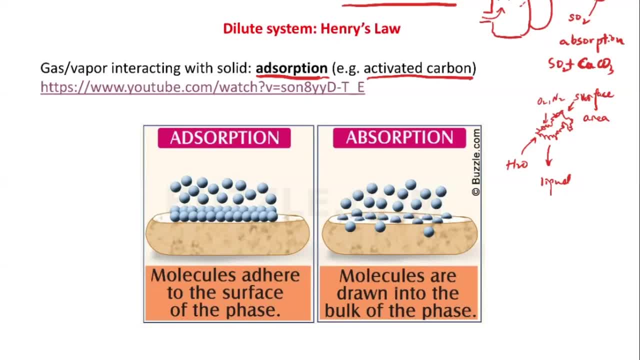 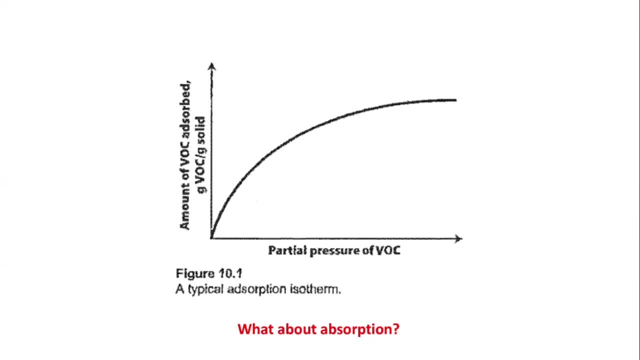 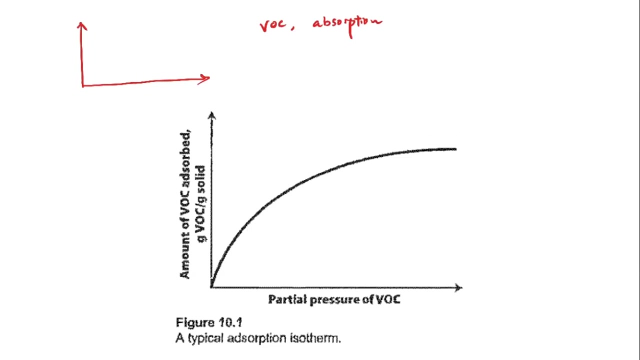 pushing these air molecules outside and forming bubbles, okay, and so we showed that. for the absorption system, let's say if we want to, okay. so if we want to remove VOCs with the absorption, okay. so we mentioned that the amount of the VOCs that's emitted, that's removed. 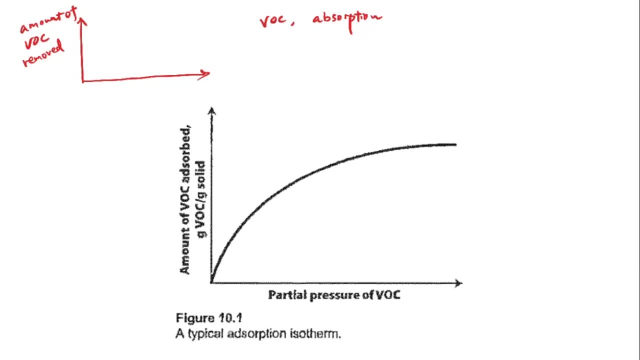 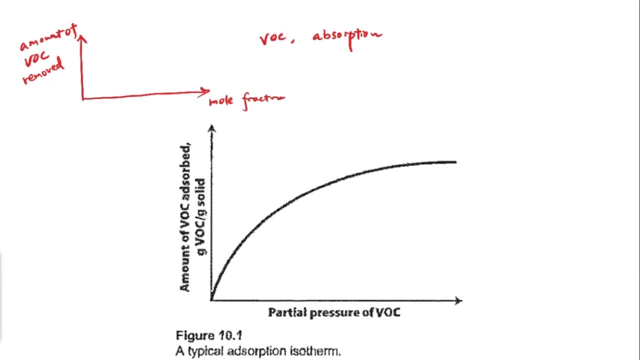 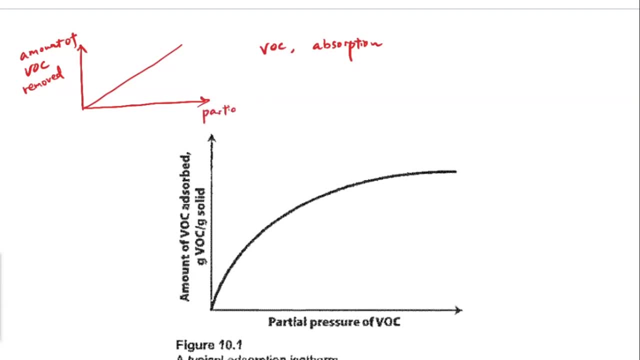 okay, you can plot it against the mole fraction. you can generally see that, because of the Henry's law, this is going to be a linear relationship. right, it shouldn't be mole fraction, it should be the partial pressure. okay, you can plot it against the mole fraction. you can generally see that, because of the Henry's law, this is going to be a linear relationship. right, it shouldn't be mole fraction, it should be the partial pressure. okay, you can plot it against the mole fraction. you can generally see that, because of the Henry's law, this is going to be a linear relationship. right, it shouldn't be mole fraction, it should be the partial pressure. okay, you can plot it against the mole fraction. you can generally see that, because of the Henry's law, this is going to be a linear relationship. right, it shouldn't be mole fraction, it should be the partial pressure. so basically, the more 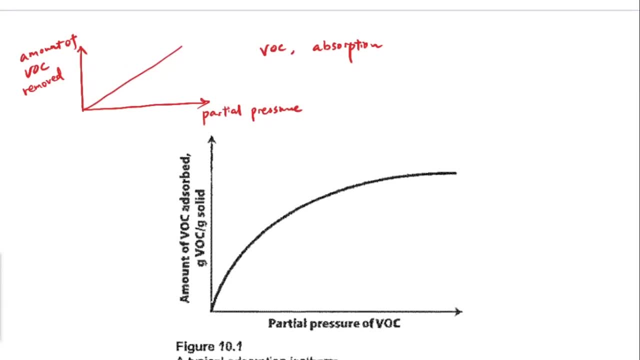 so, basically, the more so, basically, the more voces we put in the flue gas, voces we put in the flue gas, voces we put in the flue gas, the more vocs we're going to get absorbed. and this is according to the Henry's law. 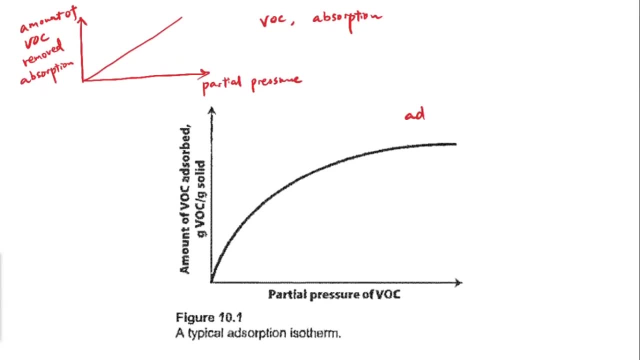 and this is according to the Henry's law, and this is according to the Henry's law, but for, but for the but for, but for the but for, but for the disruption. things will be quite different mainly. things will be quite different mainly. things will be quite different mainly because 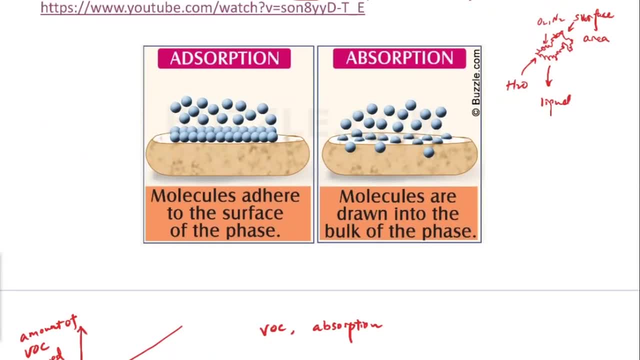 because, because for the active carbon. you only have this for the active carbon, you only have this for the active carbon. you only have this large of a surface area, right. you cannot large of a surface area, right. you cannot large of a surface area, right. you cannot infinitely add. 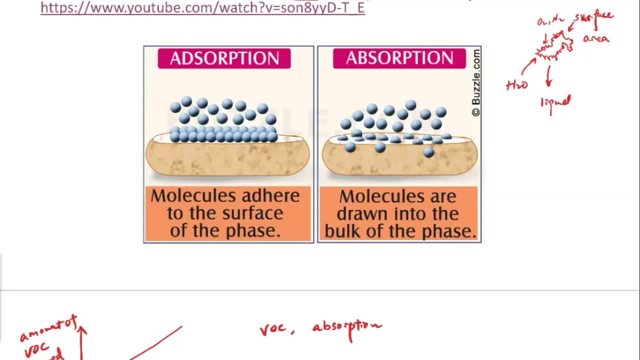 infinitely add, infinitely add. amount of amount of amount of, uh, uh, uh. add the vocs onto the surface. okay, so add the vocs onto the surface. okay, so add the vocs onto the surface. okay, so there's always a limit, there's always a limit, there's always a limit. so that's why, if we consider the amount, 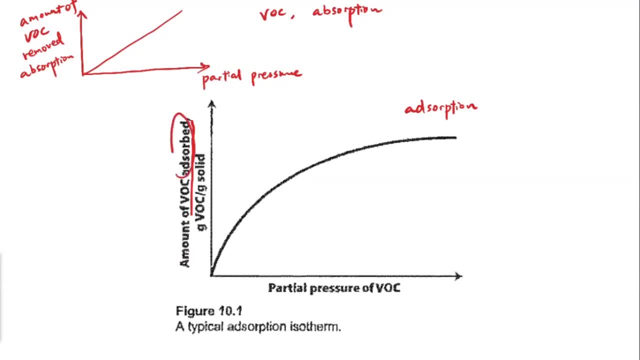 so that's why, if we consider the amount, so that's why, if we consider the amount of vocs, of vocs, of vocs getting absorbed, you're all you're always going to see, you're all you're always going to see, you're all you're always going to see this curved shape here. okay. 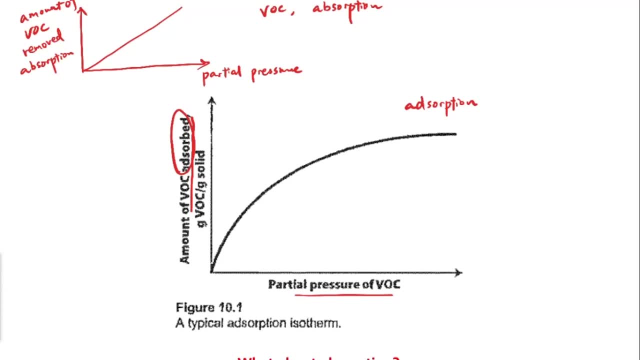 this curved shape here, okay, this curved shape here, okay. so basically the partial pressure when. so, basically the partial pressure when. so basically the partial pressure when it first increases, you're going to see a it first increases, you're going to see a it first increases. you're going to see a linear relationship here, mainly because 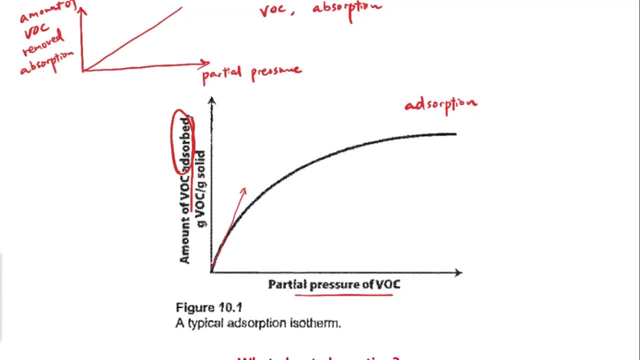 linear relationship here, mainly because linear relationship here, mainly because the active carbon are still very clean. the active carbon are still very clean. the active carbon are still very clean on its surface, but as you further add on its surface, but as you further add on its surface, but as you further add more vocs into the system, 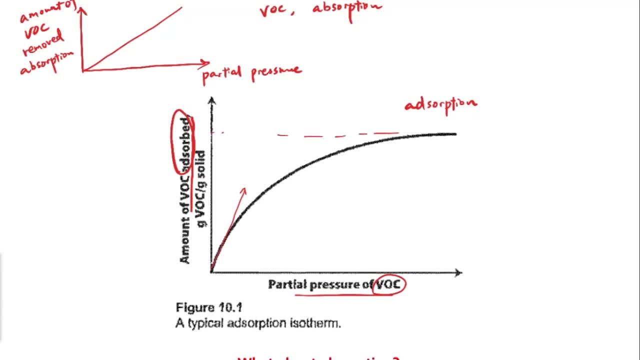 more vocs into the system, more vocs into the system, then you're going to see that at some. then you're going to see that at some. then you're going to see that at some point, point, point, there's going to be a saturation. there's going to be a saturation. 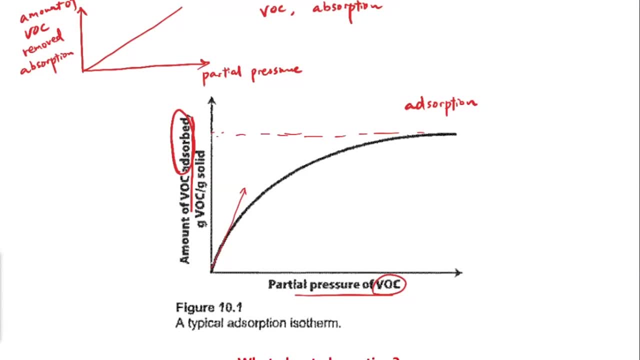 there's going to be a saturation, and what this means is that is that, and what this means is that is that, and what this means is that is that once the active carbon is saturated, we, once the active carbon is saturated, we, once the active carbon is saturated, we cannot absorb any more vocs, we cannot. 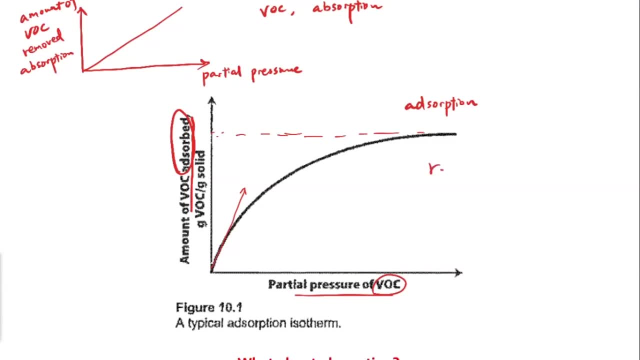 cannot absorb any more vocs. we cannot, cannot absorb any more vocs. we cannot remove the vocs anymore. okay, so we have remove the vocs anymore. okay, so we have remove the vocs anymore. okay, so we have to regenerate, to regenerate, to regenerate these, uh, active carbon. 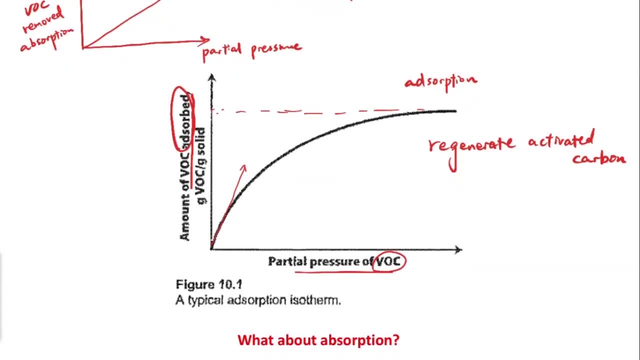 so we can um commonly regenerate the. so we can um commonly regenerate the. so we can um commonly regenerate the active carbon by just heating them up. active carbon by just heating them up. active carbon by just heating them up. okay, let's say we have this active. okay, let's say we have this active. 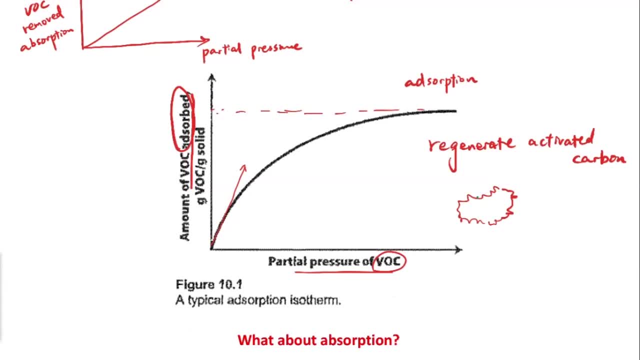 okay, let's say, we have this active carbon here, carbon here, carbon here, and it's attached with some voc and it's attached with some voc and it's attached with some voc. molecules, molecules, molecules, a lot of them, molecules, a lot of them, molecules, a lot of them on the surface right. 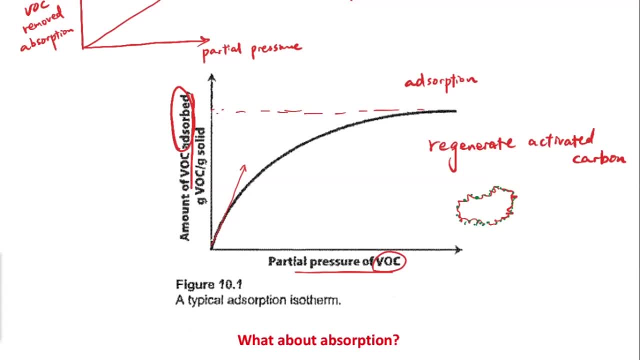 on the surface right on the surface right. because we have too much. that means that, because we have too much, that means that, because we have too much, that means that we're already probably at this point, we're already probably at this point, we're already probably at this point. here we cannot absorb more voc molecules. 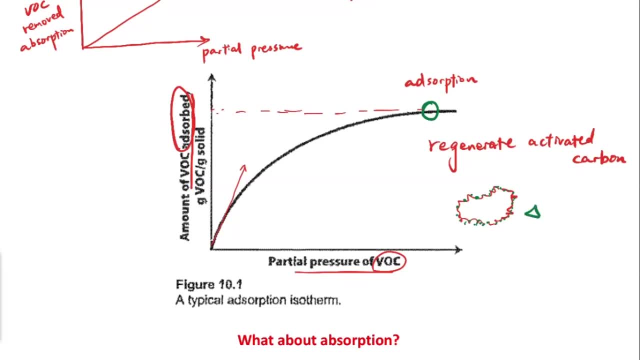 here we cannot absorb more voc molecules, here we cannot absorb more voc molecules. and under this situation we can just, and under this situation, we can just, and under this situation, we can just warm it up right by heating, warm it up right by heating, warm it up right by heating, and then we can. 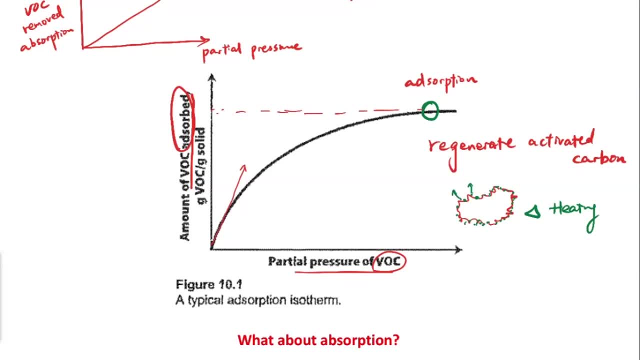 and then we can, and then we can basically vaporize all of these vocs, basically vaporize all of these vocs, basically vaporize all of these vocs back into the um, let's say a container, back into the um, let's say a container- back into the um, let's say a container or a um or a side stream. okay, so for or a um or a side stream. okay, so for. or a um or a side stream. okay, so for that side stream, that side stream, that side stream. it's going to have more vocs and we can. it's going to have more vocs and we can. 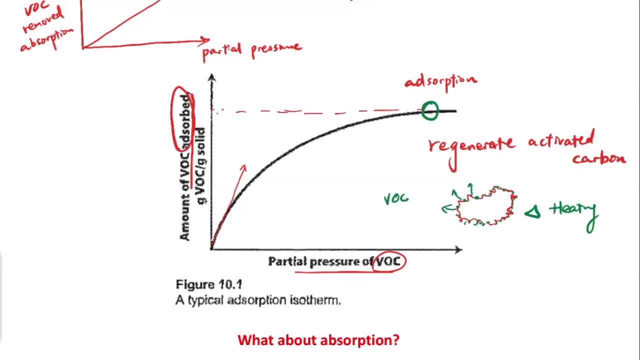 it's going to have more vocs and we can process them either by condensation or process them either by condensation or process them either by condensation or by by by other reaction processes. so you can see other reaction processes. so you can see other reaction processes. so you can see that the activated carbon 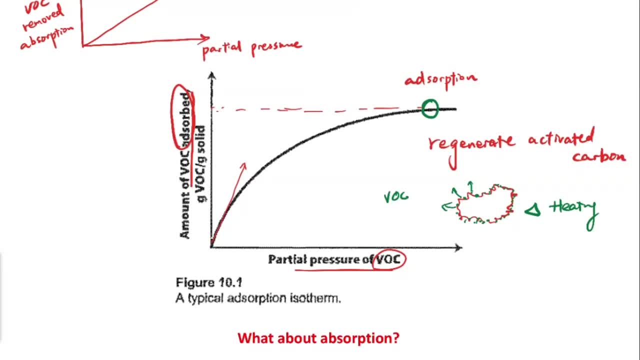 that the activated carbon, that the activated carbon. the problem for that is um, the problem for that is um, the problem for that is um. you always, you always have to regenerate, you always, you always have to regenerate, you always, you always have to regenerate them, so, them. so, if you use active carbon for the removal 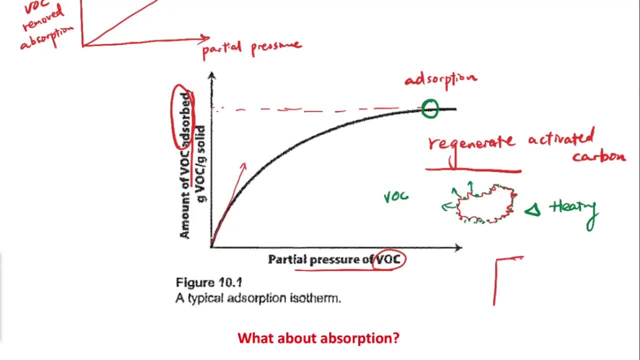 if you use active carbon for the removal, if you use active carbon for the removal of the voc, of the voc of the voc. let's say you design a control system. let's say you design a control system. let's say you design a control system that's packed with all of these active. 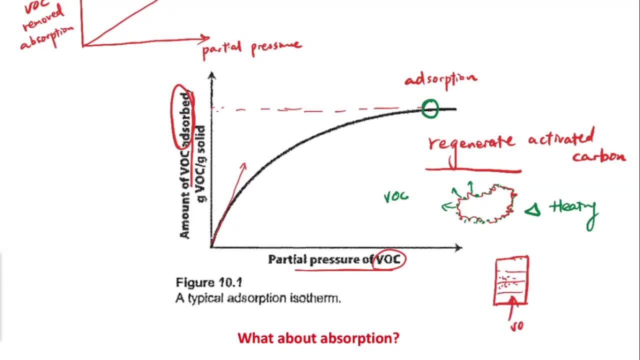 that's packed with all of these active, that's packed with all of these active, carbon, carbon, carbon, right, and then you introduce the vocs right, and then you introduce the vocs right, and then you introduce the vocs to get it purified, to get it purified. 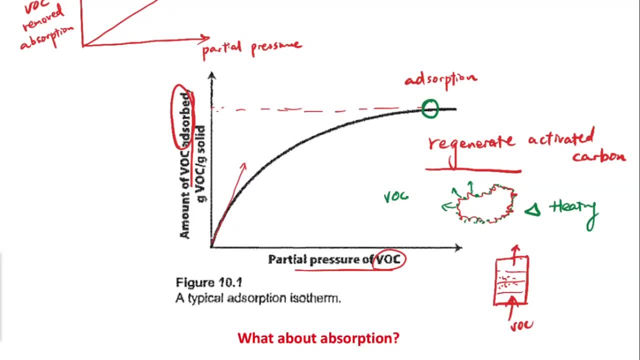 to get it purified. it's going to be similar to the back. it's going to be similar to the back. it's going to be similar to the back. house, house, house, future system- right, you need to future system. right. you need to future system. right, you need to take it offline after a certain time of. 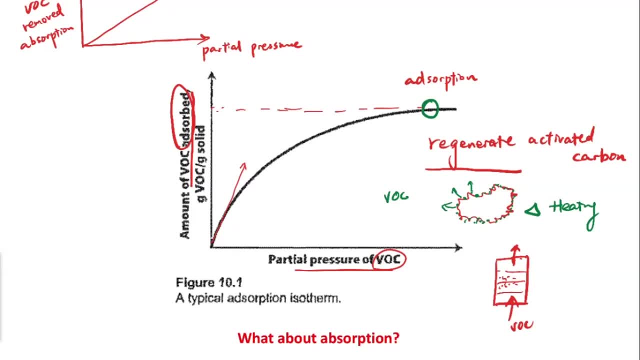 take it offline after a certain time of take it offline after a certain time of operation. because operation, because operation, because once it hits the saturation, once it hits the saturation, once it hits the saturation, you're not going to process more vocs, you're not going to process more vocs. 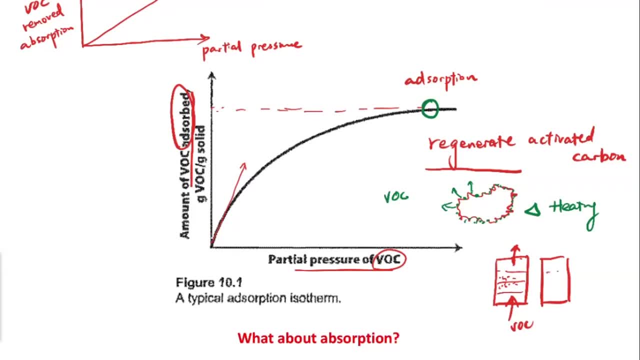 you're not going to process more vocs, so that's why you always need to design. so that's why you always need to design, so that's why you always need to design. extras, extras, extras. generally. just one more extra of the generally. just one more extra of the. 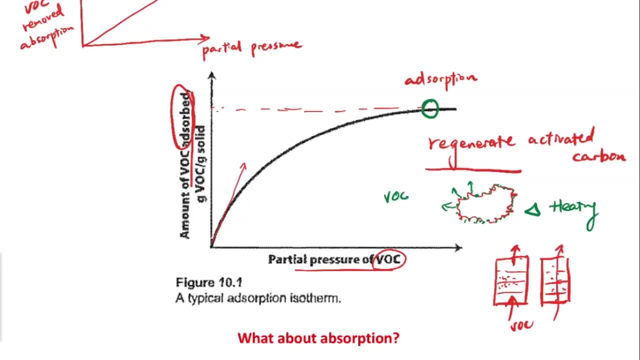 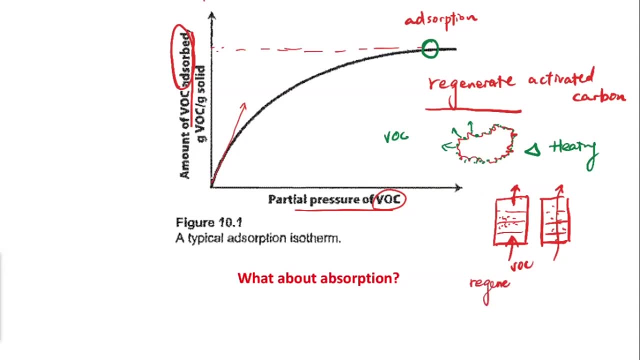 generally, just one more extra of the absorber: absorber, absorber, right, right, right. so, while this is being so, while this is being so, while this is being here, the active carbon is being here, the active carbon is being here, the active carbon is being regenerated, and this one can be put in the 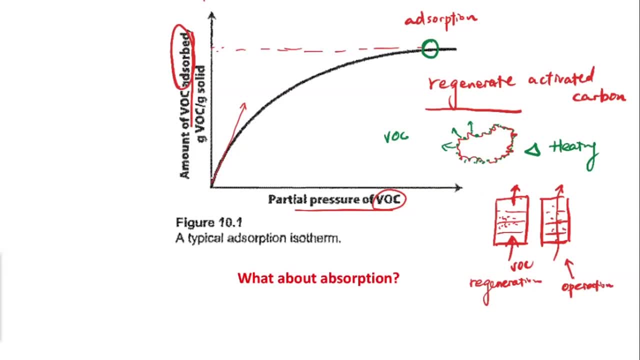 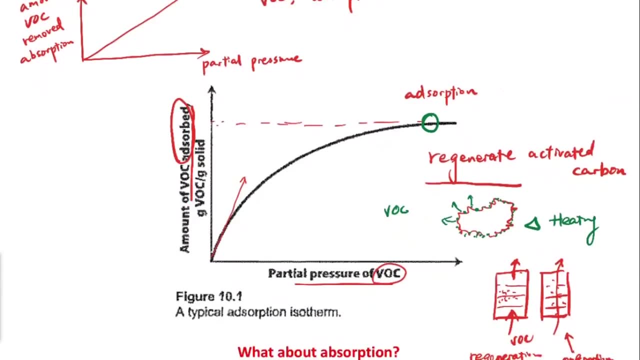 and this one can be put in the and this one can be put in the operation. okay, okay, okay. so this is the voc control with the. so this is the voc control with the. so this is the voc control with the adsorption, and later you can find how we. 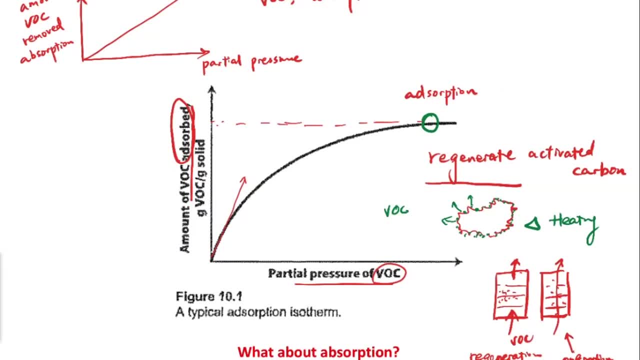 adsorption, and later you can find how we adsorption, and later you can find how we can design these, can design these, can design these voc absorbers, voc absorbers, voc absorbers to remove the, to remove the, to remove the vocs from the gas streams, and we're. 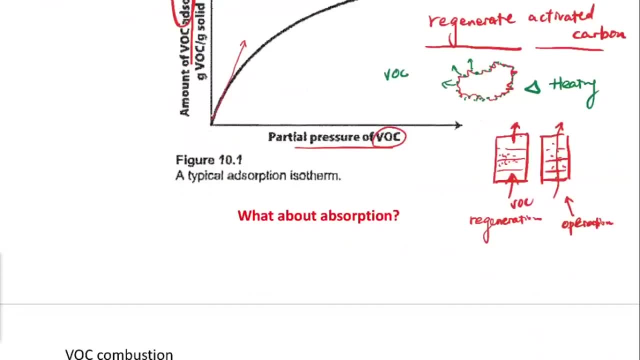 vocs from the gas streams, and we're vocs from the gas streams and we're mainly dealing with, mainly dealing with, mainly dealing with the active carbon system, the active carbon system, the active carbon system. okay, okay, okay, so we can also use the voc. so we can also use the voc. 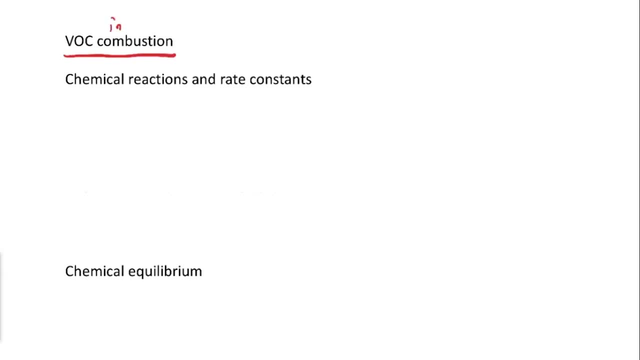 so we can also use the voc- combustion, and people also call this as combustion, and people also call this as combustion and people also call this as voc- incineration. the reason why we can combust. it is the reason why we can combust. it is the reason why we can combust. it is this. we will see the full name, if you. 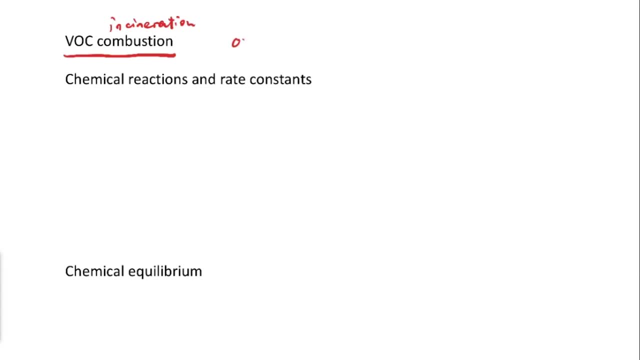 this, we will see the full name. if you this, we will see the full name. if you think about it, that's volatile organic. think about it, that's volatile organic. think about it, that's volatile organic compounds. right, which means that it's composed of carbon, which means that it's composed of carbon. 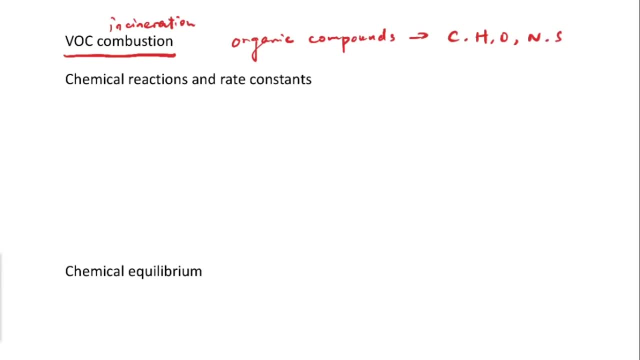 which means that it's composed of carbon, hydrogen oxygen, maybe nitrogen and hydrogen oxygen, maybe nitrogen and hydrogen oxygen, maybe nitrogen and sulfur inside, sulfur inside, sulfur inside, which means that they can be, which means that they can be, which means that they can be combustible, combustible. 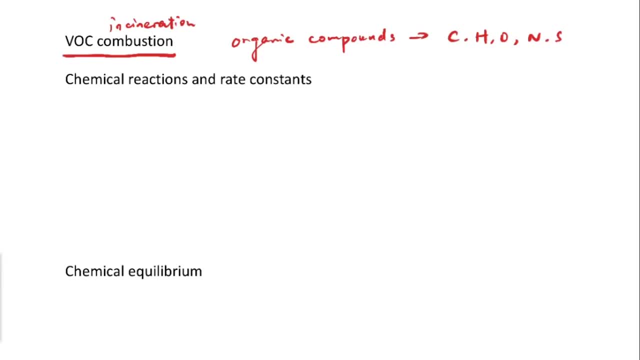 combustible, so we can basically just add in air, and so we can basically just add in air, and so we can basically just add in air and then then then put it at a high temperature that oxygen, put it at a high temperature that oxygen, put it at a high temperature that oxygen to. 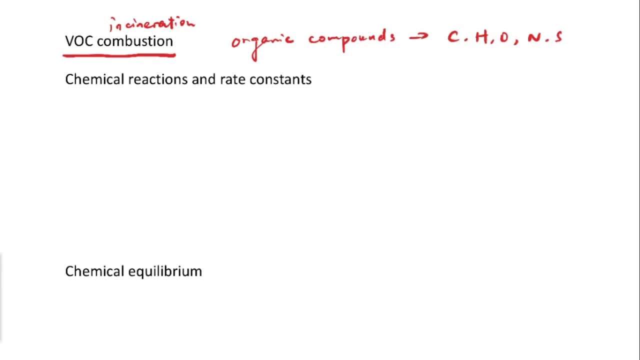 to to react with these vocs and get them react with these vocs and get them react with these vocs and get them removed, removed, removed, okay, and here i just want to briefly okay, and here i just want to briefly okay, and here i just want to briefly review some of your. 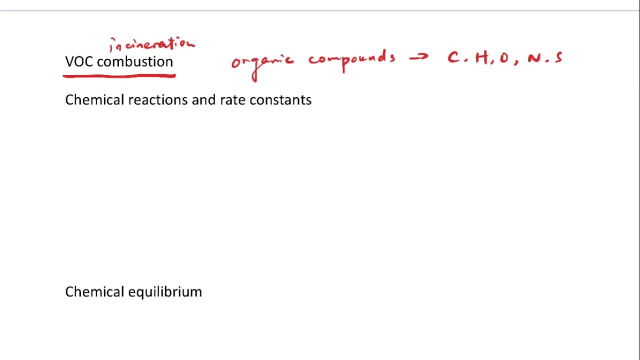 review some of your review, some of your important, some of the important concepts important. some of the important concepts important, some of the important concepts in the reaction engineering, in the reaction engineering, in the reaction engineering. okay so in terms of the voc combustion. okay so in terms of the voc combustion. 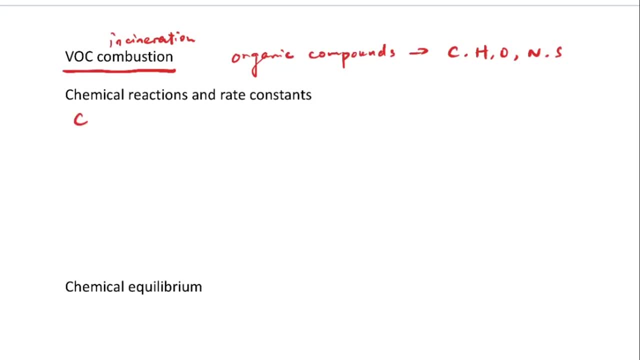 okay. so in terms of the voc: combustion, it involves, generally involves chemical. it involves, generally involves chemical. it involves, generally involves chemical reactions: okay so when we talk about the sulfur: okay. so when we talk about the sulfur, okay. so when we talk about the sulfur dioxide control, we already 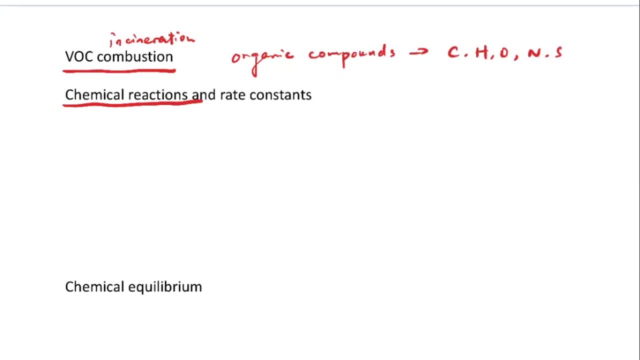 dioxide control- we already dioxide control. we already mentioned something. or nitrogen dioxide mentioned something. or nitrogen dioxide mentioned something. or nitrogen dioxide control- we already mentioned something. control: we already mentioned something. control- we already mentioned something about the reaction rates, about the reaction rates, about the reaction rates. so let's assume that reaction happening. 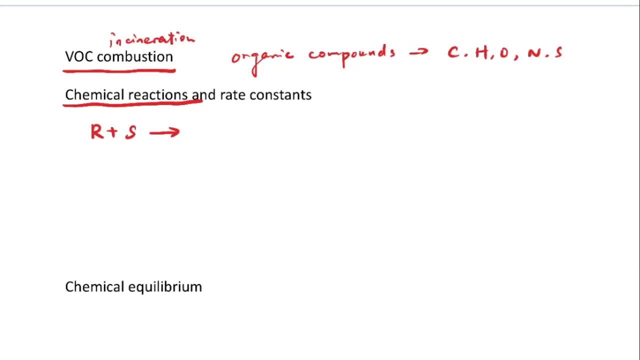 so let's assume that reaction happening. so let's assume that reaction happening between the voc and oxygen, between the voc and oxygen, between the voc and oxygen, is r plus s going to p plus q, is r plus s going to p plus q, is r plus s going to p plus q, and then we can calculate the reaction. 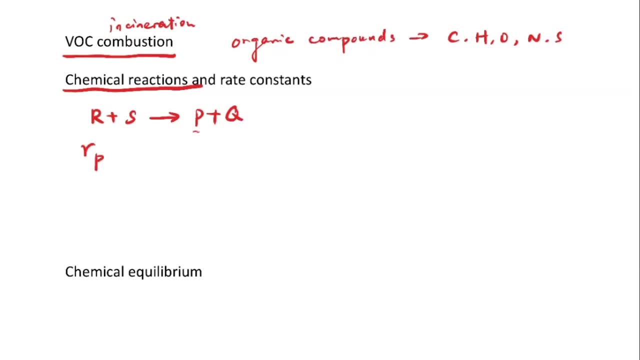 and then we can calculate the reaction, and then we can calculate the reaction rate, rate, rate. this is corresponding to for the product. this is corresponding to for the product. this is corresponding to for the product: p, p, p. it's going to be equal to k multiplied by. 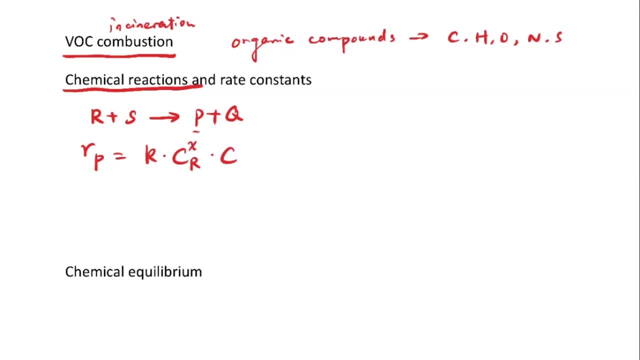 it's going to be equal to k multiplied by. it's going to be equal to k multiplied by: the concentration of r to the power x. the concentration of r to the power x. the concentration of r to the power x, multiplied by the concentration of s, multiplied by the concentration of s. 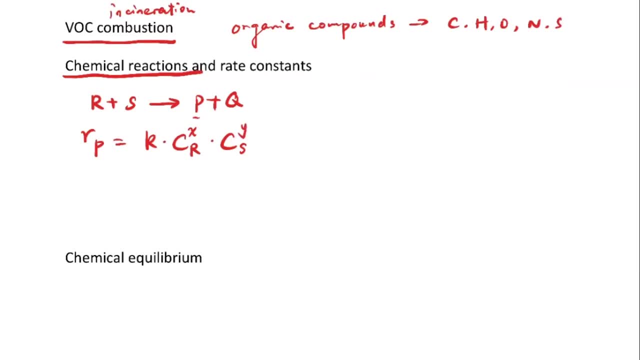 multiplied by the concentration of s to the power y to the power y to the power y. okay, so, in this, okay, so in this, okay, so in this equation, here the k equation, here, the k equation, here the k is called the rate constant. okay, so the cr and cs. 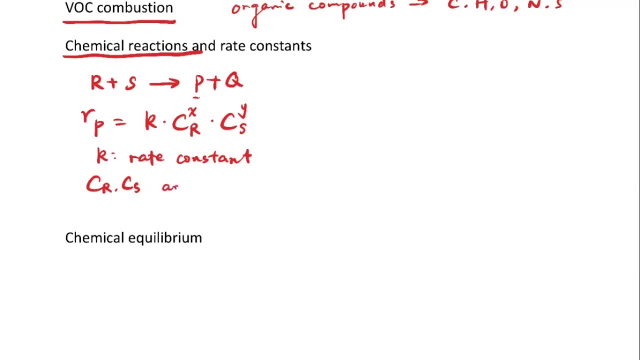 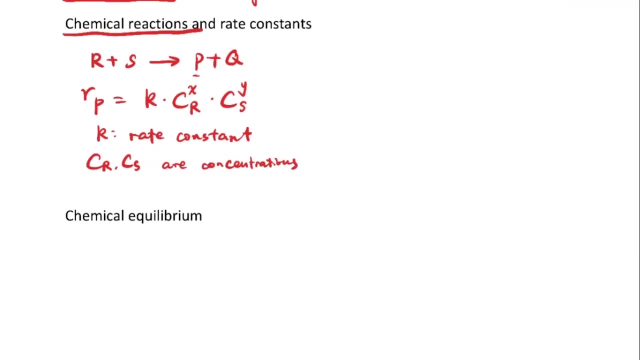 okay. so the cr and cs: okay, so the cr and cs, they are the concentrations. okay and generally we will use the unit. okay and generally we will use the unit. okay and generally we will use the unit of mole per liter or of mole per liter or of mole per liter or mole per meter cube. 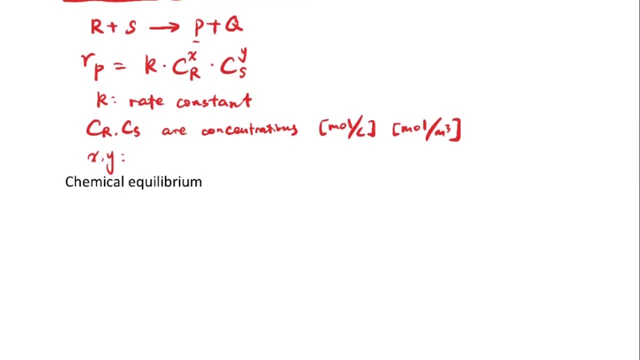 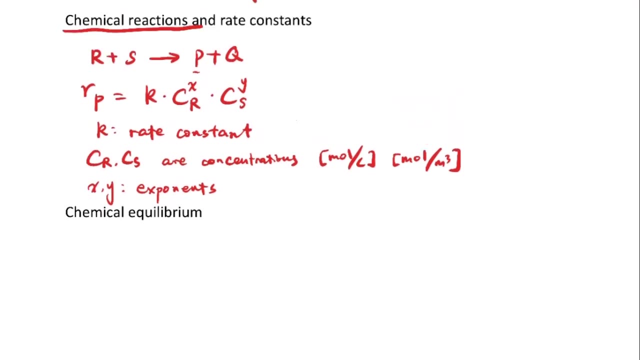 and for the x and y they are the, and for the x and y they are the, and for the x and y they are the exponents. okay, so generally, let's say if we. okay, so generally, let's say if we. okay, so generally let's say if we. if we describe, 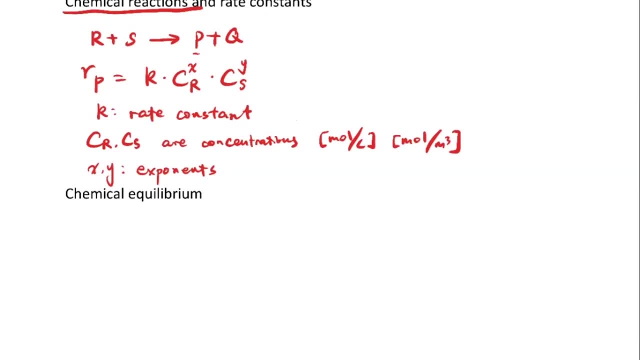 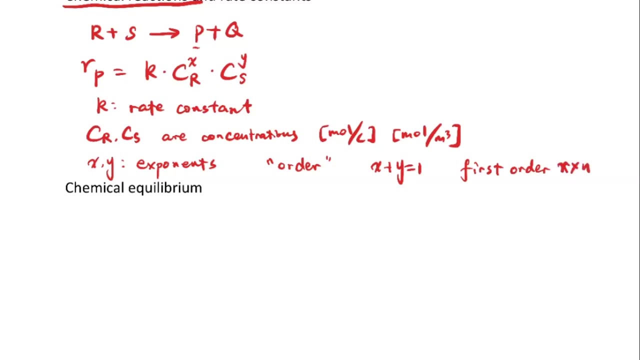 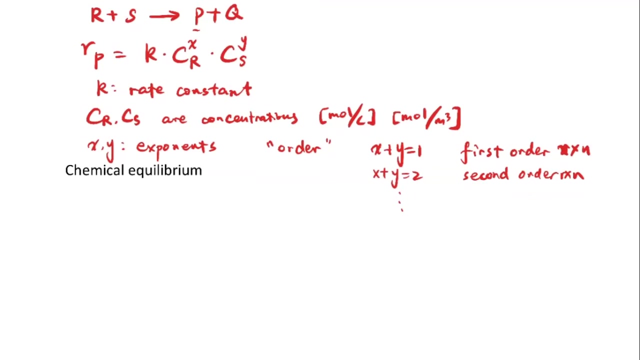 an equation, uh, if, if we describe a chemical reaction, we'll also use the term order okay. so if x plus y equal to one, we call that first order reaction okay. x plus y equal to two, that's second order okay. so on and so forth. right, so, um, and generally these x and y. so, for example: 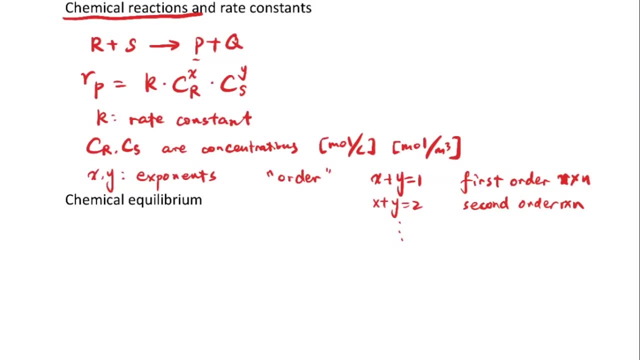 if we're talking about the elementary reaction, then normally the x and y will just be equal to the numbers, that's in front of the, the chemical in front of the reaction reactants. okay, but for a lot of the reactions the x and y have to be derived from the experiments. 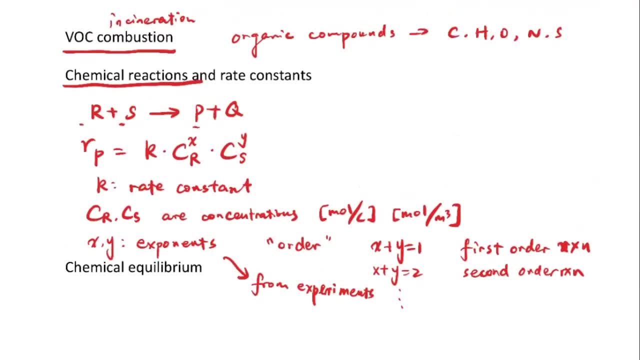 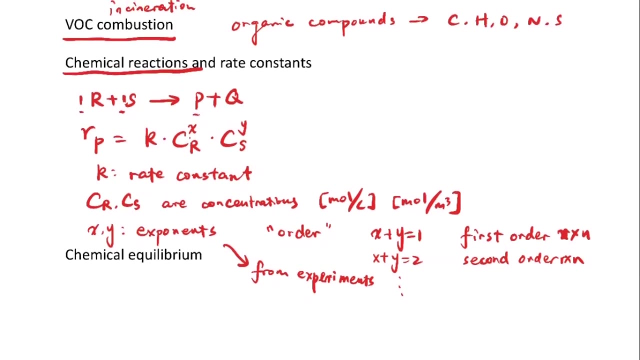 so we shouldn't take it for granted if we just see that there's one in front of r and one in front of s, so this doesn't mean that the x and y are equal to one. we have to derive the exponents from the chemical reactions. okay, so this is about the chemical reaction and further. 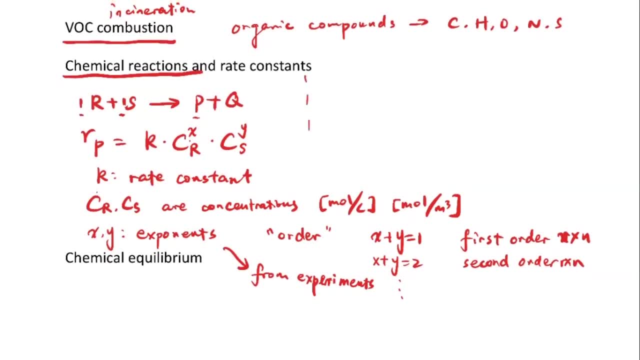 about the reaction rate constant. so if i further write it off here, so generally people will use the erroneous form of the rate constant, which is equal to k, is equal to a multiplied by exponential of e divided by rt. okay, so in this equation a is the frequency function. 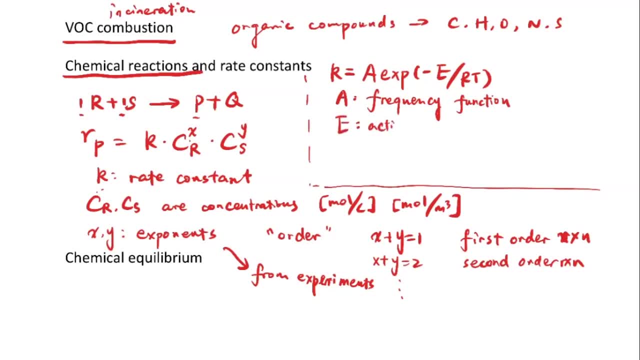 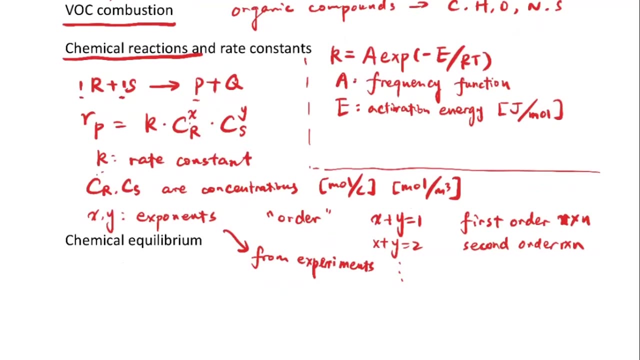 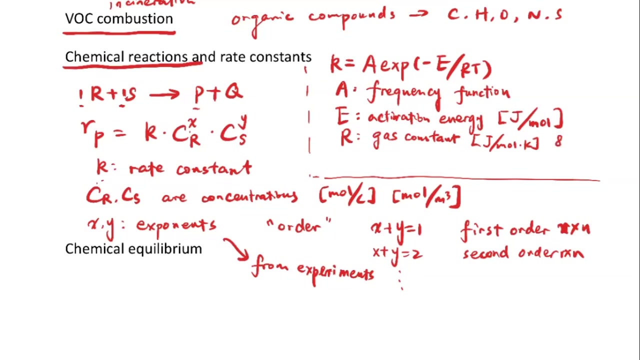 e is activation energy, okay, and this has a unit of joule per mole, and r here is the gas constant. so from the ideal gas law we know that when it's carrying a unit of joule per mole, okay. so the r is going to be 8.314, okay, and then the temperature and the t. here is the temperature. 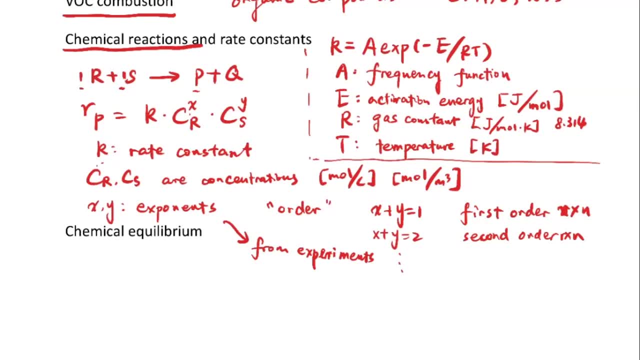 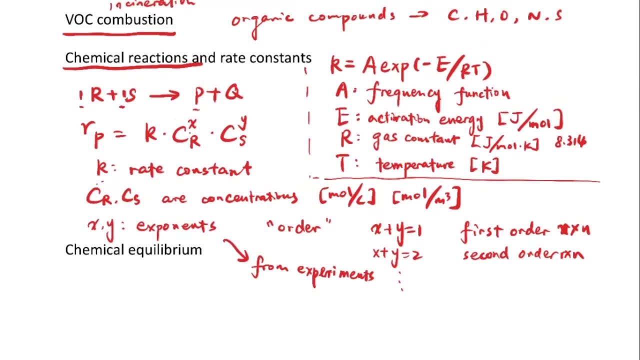 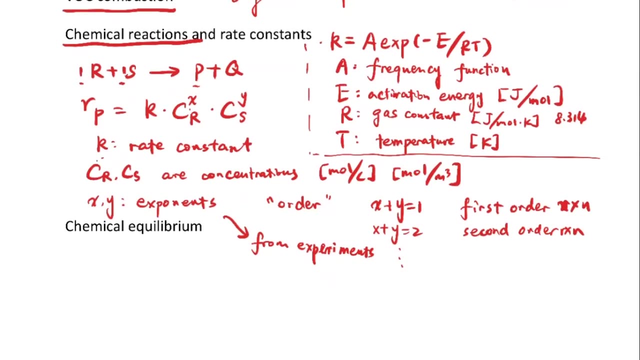 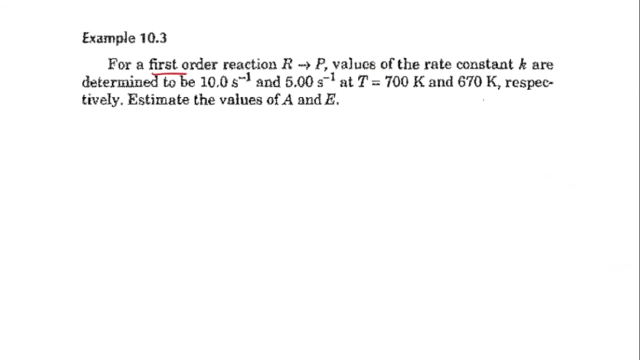 and that's going to carry a unit of kelvin. okay, so this is how we can calculate the rate constant. or we can also use this equation to derive the activation energy for certain reactions and we can also talk about the chemical equilibrium. but here i think we can first go through an example here. so let's say we have a first auto reaction. 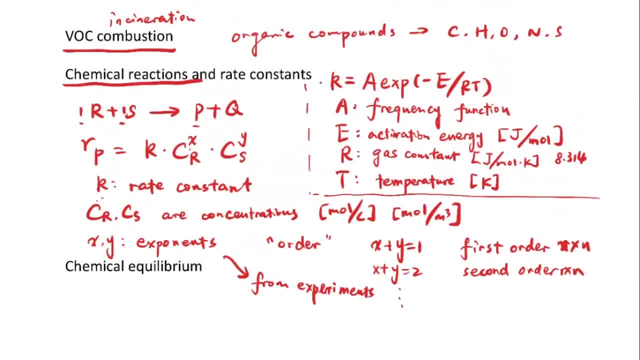 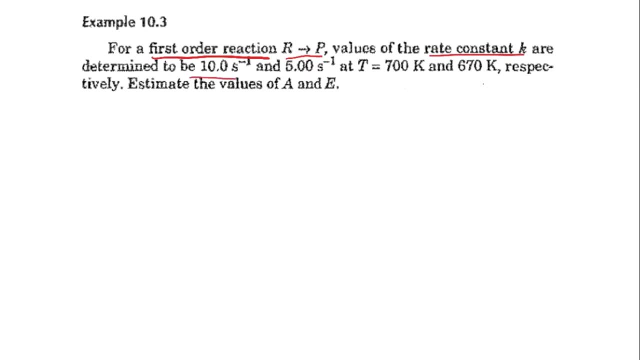 okay, r going to p, not this one. r plus s going to P, plus Q are going to P. So the rate constant K are determined to be 10 per second and five percent second at two different temperatures. And then it wants us to estimate the value of A and E. So according to the equation for the rate constant, we know that 10 or 10.0. 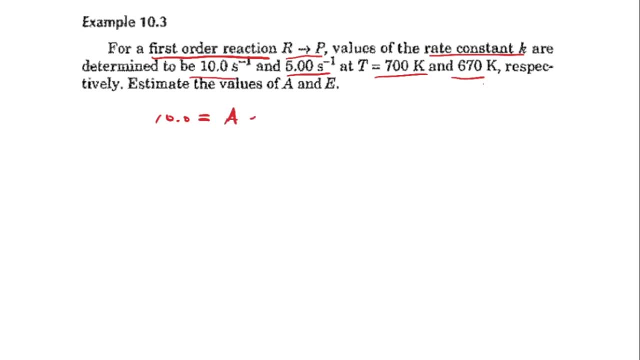 it's going to be equal to A multiplied by the exponential of minus E divided by RT. All right, and here we know that the T is basically 700 kelvin, which is A exponential minus E divided by 8.314 multiplied by 700. 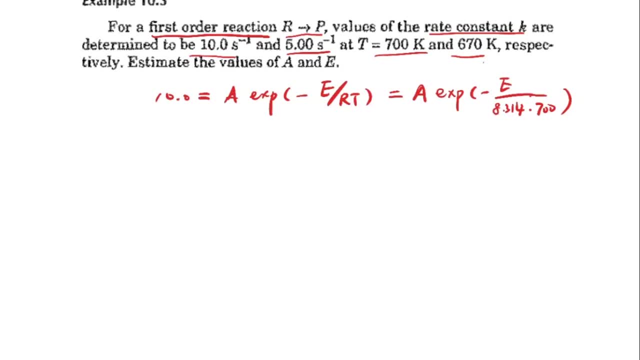 Okay, And for the second condition, we have 5.0 equal to A, multiplied by exponential of minus E, divided by 8.314 multiplied by 670.. Okay, so we have two equations, two unknowns, which are A and E. You can. 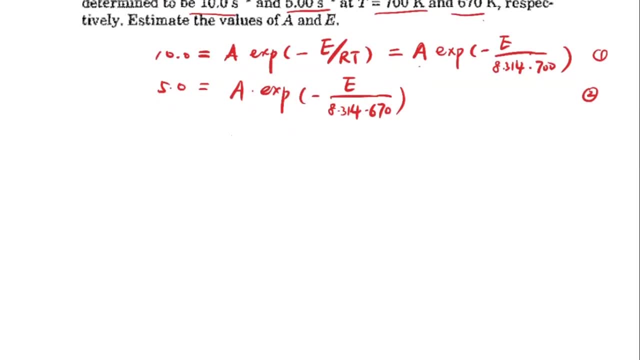 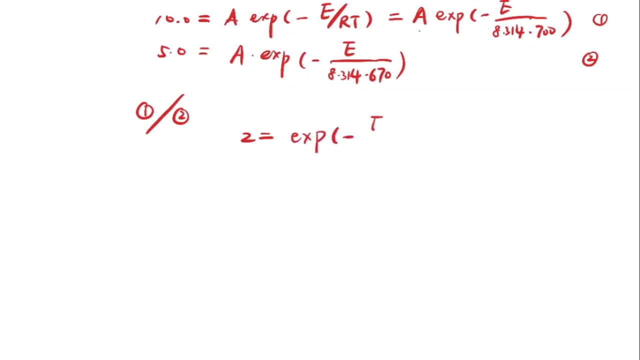 maybe first divide these two equations to get what is the E values. So if you use equations 1 divided by equation 2, then you have 2 equal to. you know, we're going to cancel out the A here. So we have exponential of minus E divided by 8.314 multiplied by 1 divided by 700, minus 1 divided by. 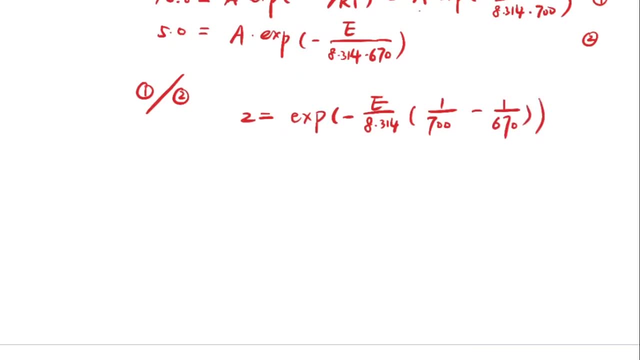 670.. Okay, So in this way you can find out basically: E is equal to nine zero zero nine two. Okay, So in this way you can find out basically: E is equal to nine zero zero nine two. Joule per mole. Joule per mole. 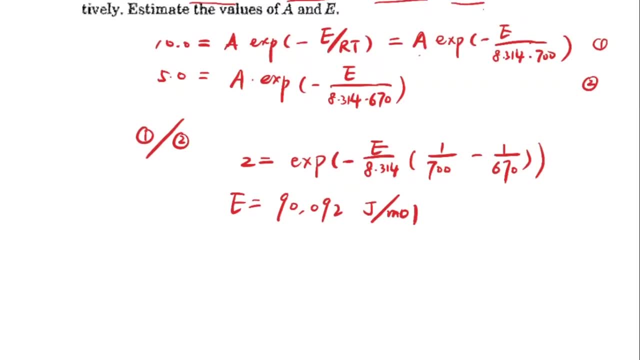 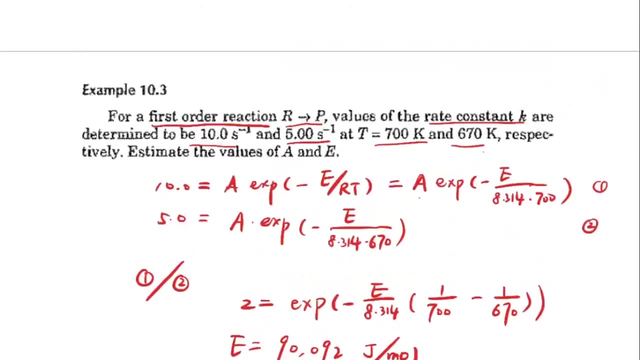 And if we have E, then you can plug in any of the equation and find out that A, the frequency factor or the frequency function, is equal to 5.28 multiplied by 10 to the seven per second. Okay, So this is how we can use the rate constants at different temperatures to calculate the 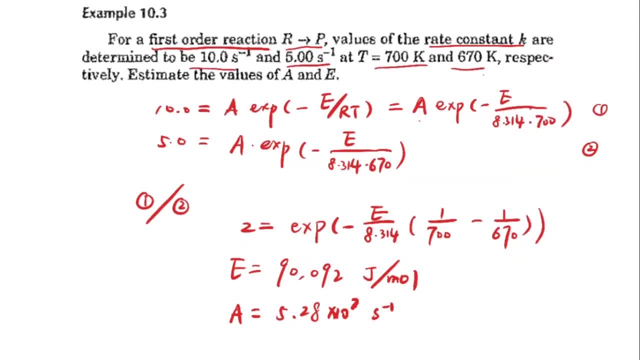 activation energy and also the frequency factor. Okay, So the first thing we need to do is to calculate the activation energy and also the frequency factor. Okay, So the first thing we need to do is to calculate the activation energy and also the frequency factor. 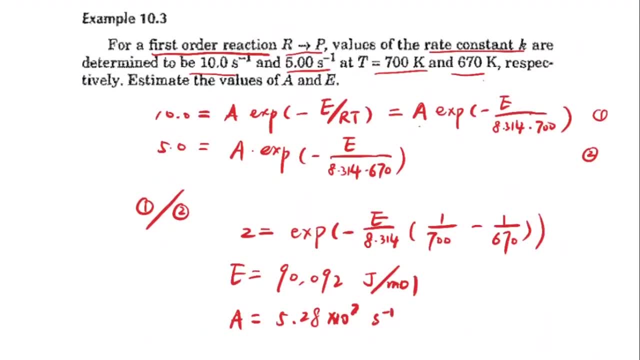 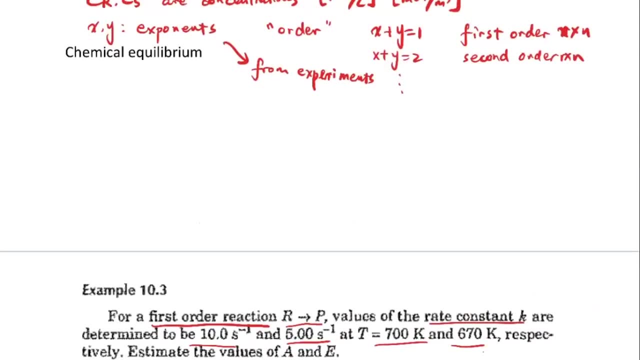 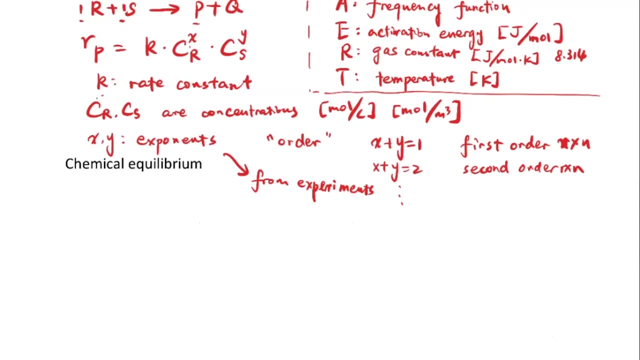 And uh, I think you probably already know this from the 261 class, but let's just do a quick review of these concepts. Okay, So if we know the chemical reaction, we can also use the chemical equilibrium. So to set up what the chemical equilibrium means is for a lot of the reactions they're not going to. 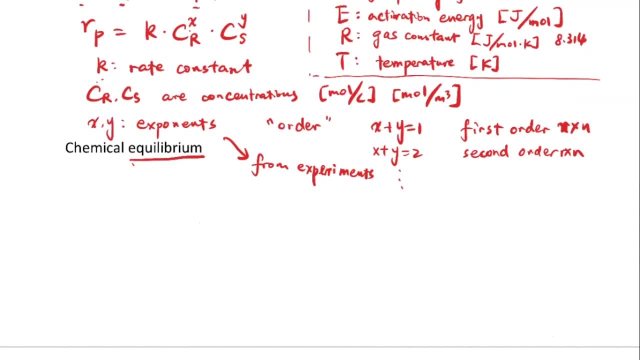 happen completely, which means that there are always going to be some reactants, some products that are being mixing or mixed inside the system. So if we just use the reaction of sulfur dioxide and oxygen as an example, okay, So we know that this example, this reaction, is reversible. 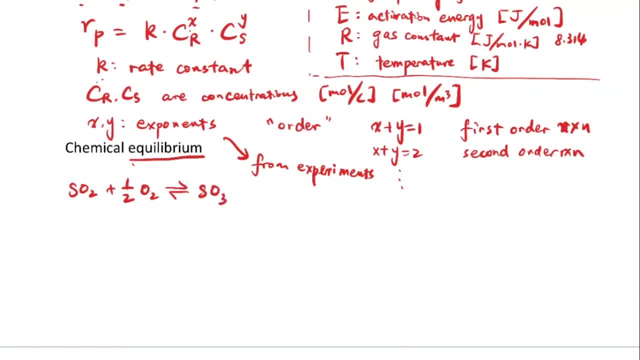 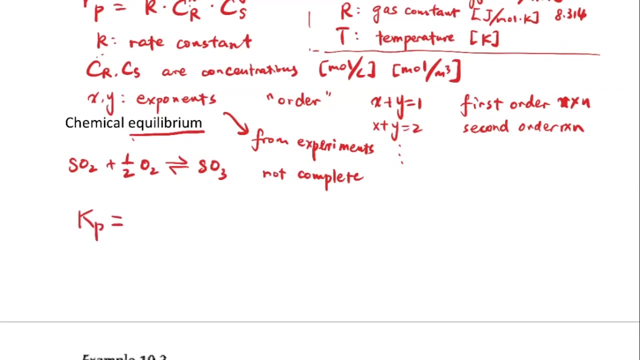 which means that they're going to form sulfur trioxide, So the reaction is not complete. Okay, so we can determine a equilibrium constant, KP, which is equal to the partial pressure of the sulfur trioxide divided by the partial pressure of sulfur dioxide multiplied by this partial pressure. 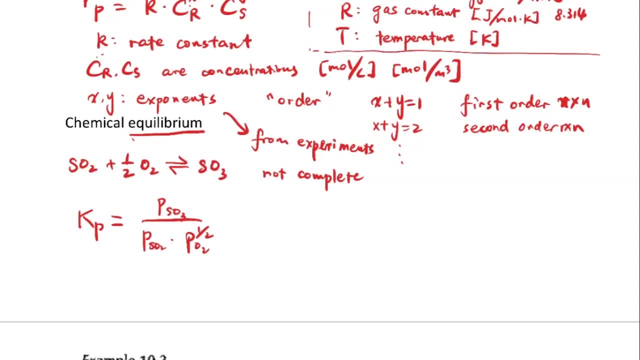 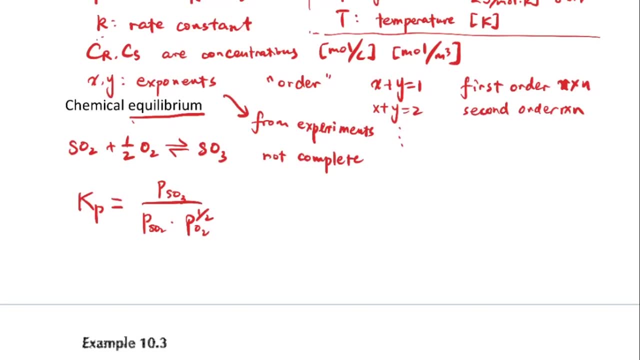 of oxygen to the power of one over two. okay, So basically what this means is that the ratio among these three factors are going to be a constant under a certain temperature. Okay, let's say a certain temperature, TC. Okay. so basically we can use this equilibrium constant. 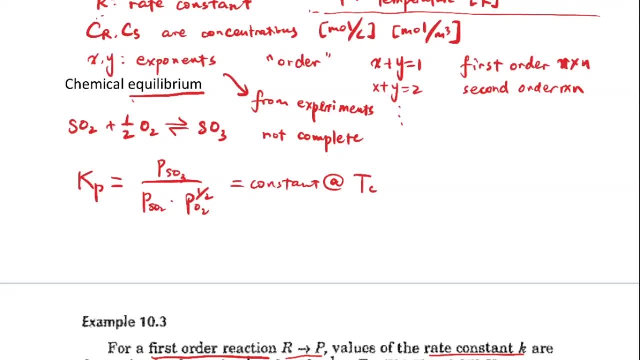 to calculate what is the concentration of certain species. Let's say, if we already know what is the concentration of sulfur, Okay, so we can use this equilibrium constant to calculate what is the concentration of sulfur trioxide. to calculate what is the concentration of sulfur trioxide. 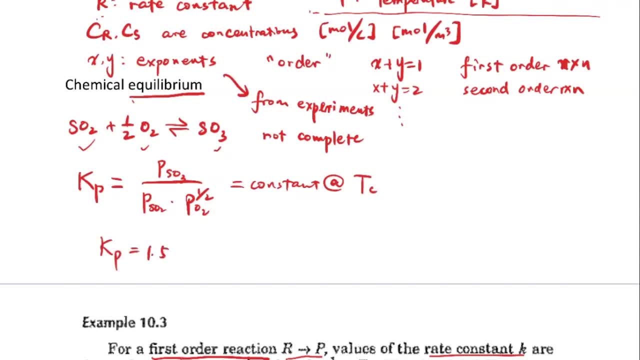 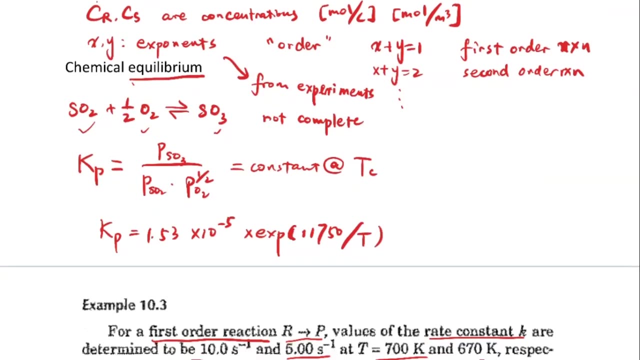 If you're interested. this rate constant is equal to 1.53 multiplied by 10, to the negative five multiplied by exponential of 11750 divided by T. Okay, so we can use this equation to determine what are the concentrations of all of the reactants. 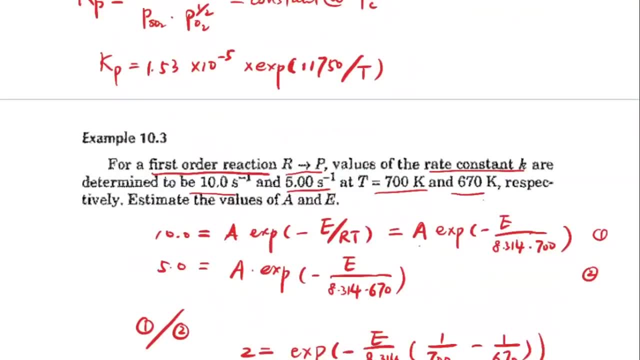 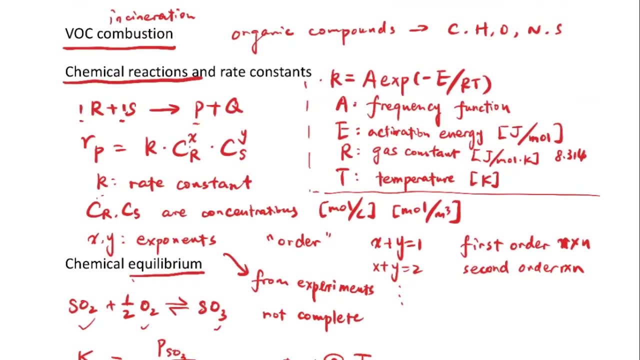 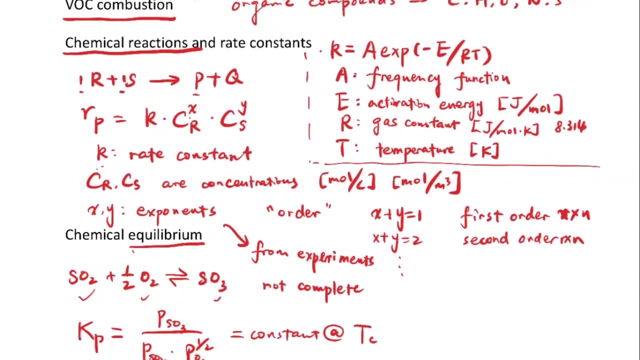 and products in certain systems. Okay, so this is the basically the removal of the VOC. We can remove these VOC by chemical reactions And generally we have to deal with the rate constants and the chemical equilibrium. So, finally, we can remove the VOCs by catalytic reactions. 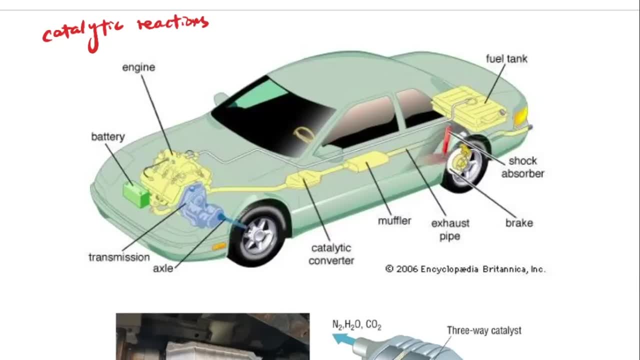 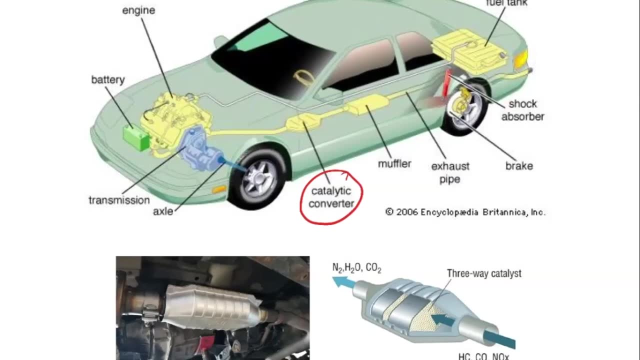 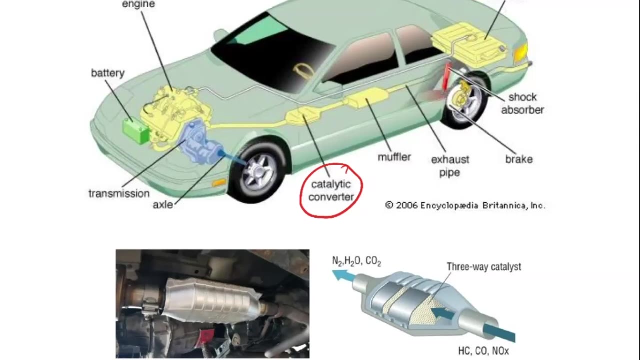 So for your cars or for your vehicles, we know that there's an important component that's called the catalytic converter. Okay, so the reason for that is when we combust the gas, let's say the gasoline, as I mentioned from the NOx control right.